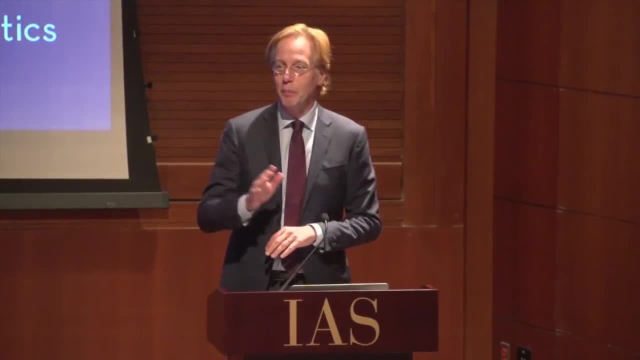 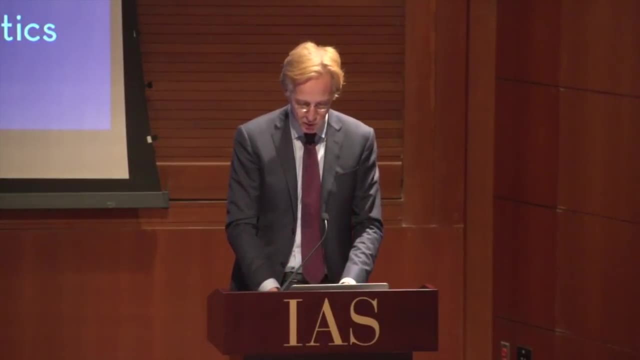 It often feels a little bit like the Olympics and you can kind of peak wrong, but Axé received the gold medal, so to say. I'd like to quote one part of the recognition of the Fields Medal committee. This highest honor recognized Axé's contribution to an exceptionally broad 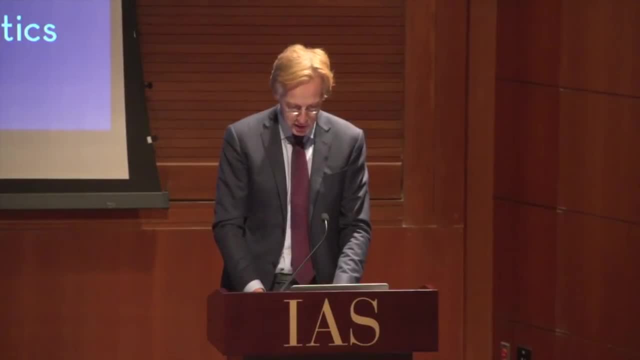 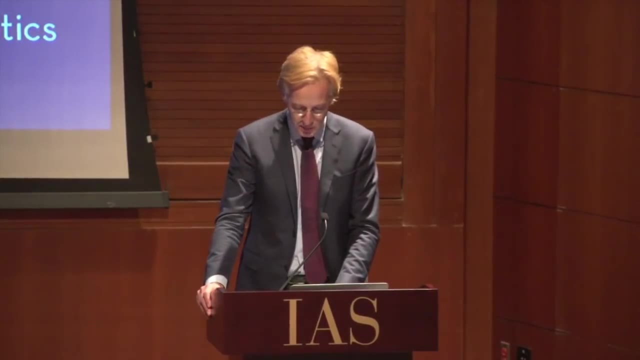 range of subjects in mathematics, including number theory, homogeneous dynamics, representation theory and arithmetic geometry. He solved many long-standing problems, including the use of methods, by combining methods from seemingly unrelated areas, presented novel viewpoints on classical problems and produced strikingly far-reaching conjectures. 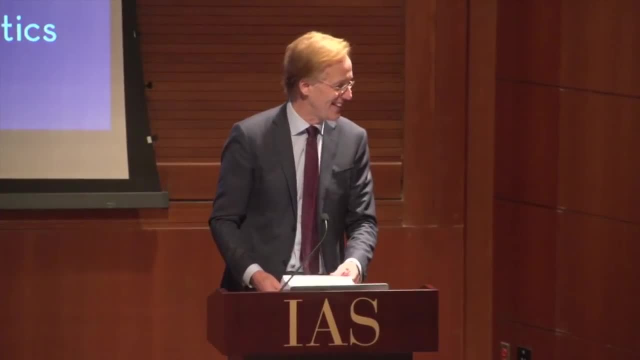 It looks like a very good description of a one-man band, so we can dismiss the rest of the faculty in the School of Maths now. Axé has, although he's quite young, a long record of advanced learning, so to speak. He by age 16,. he earned his bachelor degree in mathematics and physics at the University. 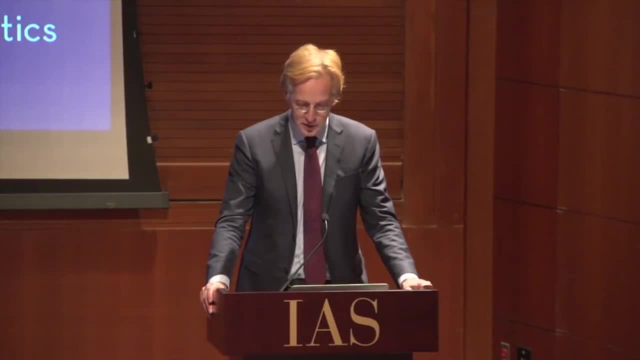 of Western Australia, and at age 20, he had already earned a PhD in mathematics at Princeton University. There are many connections to the institute. His thesis advisor at Princeton was Peter Sarnak, now a fellow professor at the institute, and Manjul Bhargava, a beloved 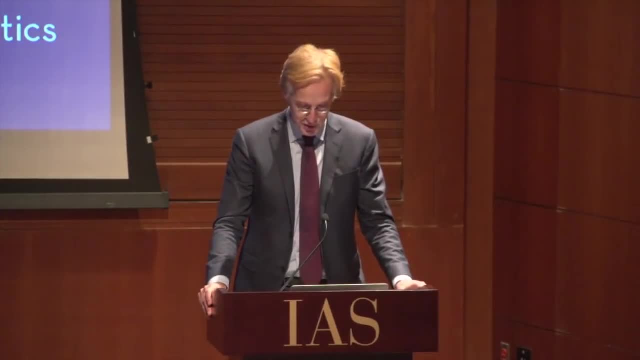 colleague and co-Fields medalist at the university was in the same graduate class, I think right, And so he was a very good friend of mine. He was a very good friend of mine And he did the research, So he was something right at that moment in that particular class. 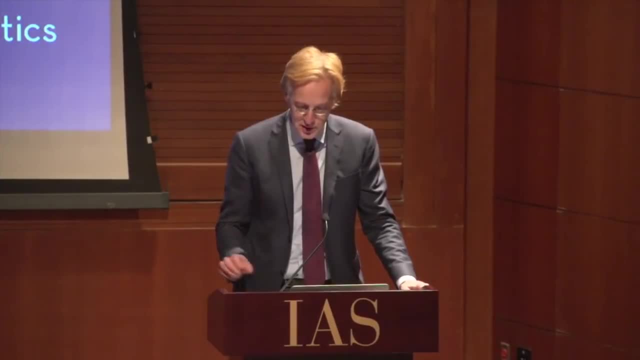 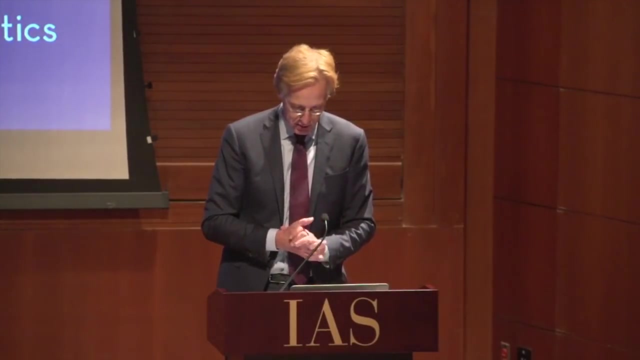 and is now a trustee of the institute. Axé came first to the institute as a member in 2005,, and he returned as a distinguished visiting professor in the 2017-2018 year to lead the special programme on analytical and topological aspects of locally symmetric spaces. 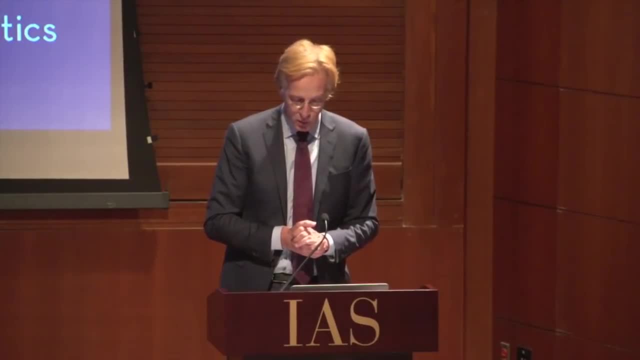 He had helped many other positions at MIT, at NYU Courant Institute of Mathematical Sciences. coming here he was at Stanford. There are many other honors. Last spring you were elected a Fellow of the Royal Society. In August he received an honorary doctorate from his 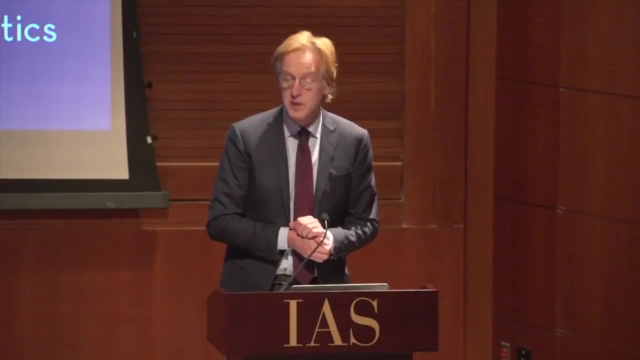 alma mater, the University of Western Australia, And during his acceptance speech that I very much enjoyed, he spoke, I would say, very eloquently about the long term of this kind of type of curiosity-driven research that the Institute stands for, I must say actually. 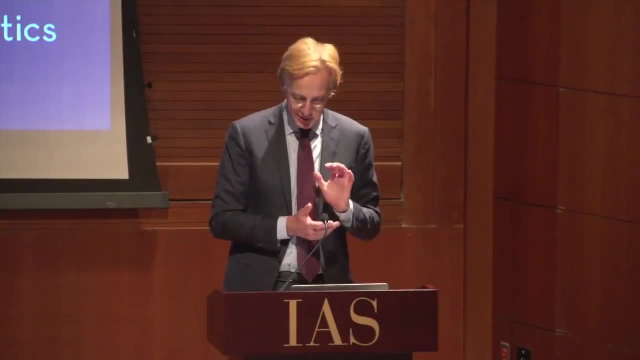 you're also a wonderful collaborator and I feel a little guilty because of course we want you to come here and devote all your attention to mathematics. but you have been also a very, very collaborative and collegial member of the Institute community, doing many 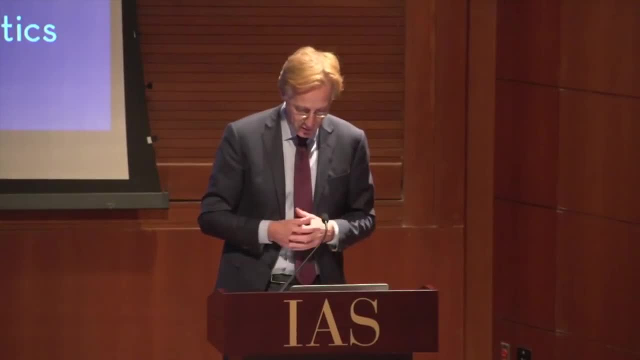 other things, a member of the Diversity Committee and, in so many ways, contributing to life at the Institute, So I want to thank you for that. It's also a great pleasure to have your wife, Sarah, and your small family. Thank you for being here and thank you for providing us tonight with your public lecture. 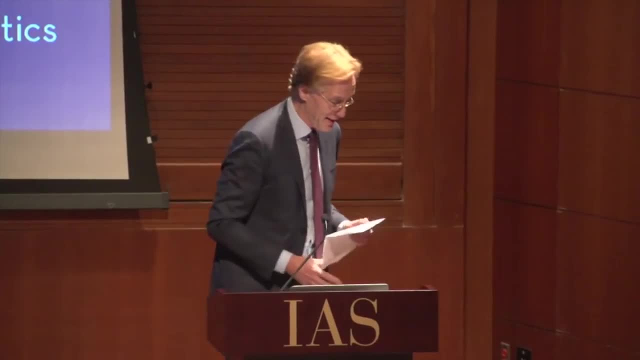 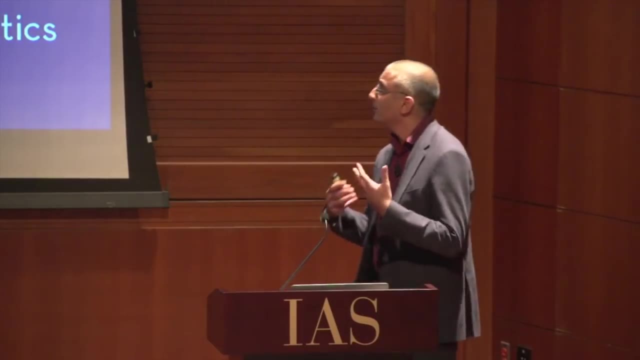 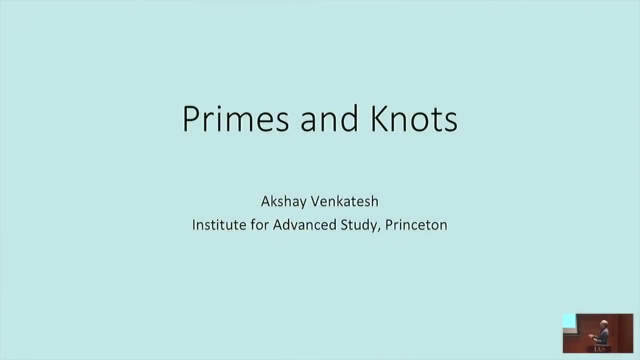 entitled Primes and Nots. Ladies and gentlemen, Axel Venkatesh. So my lecture today is about one of the, I would say, fundamental metaphors in number theory, And okay. So this, This metaphor or analogy, is that there's a very deep and interesting relationship between 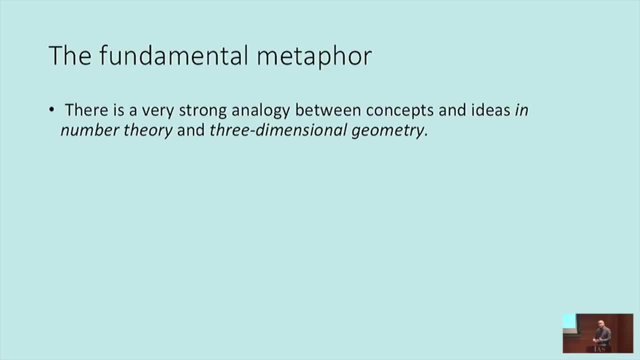 concepts in number theory, and I'll say: number theory means the arithmetic of whole numbers, but I'll say in a moment more exactly what we're going to talk about, So that on the one hand, and on the other hand, geometry in three dimensions. Okay, So this is a broad 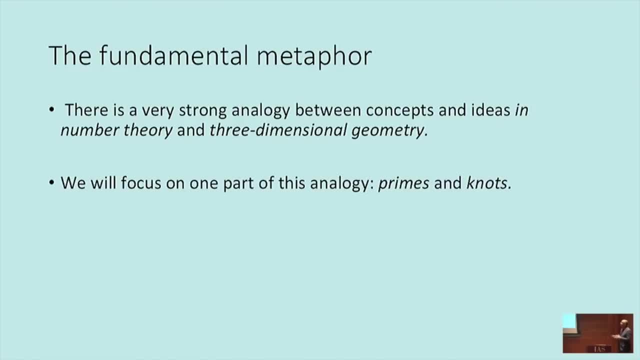 and very powerful analogy, And in the talk today I'm just going to talk about one part of it. So on the side of number theory I'll talk about prime numbers And on the side of geometry we'll talk about knots. 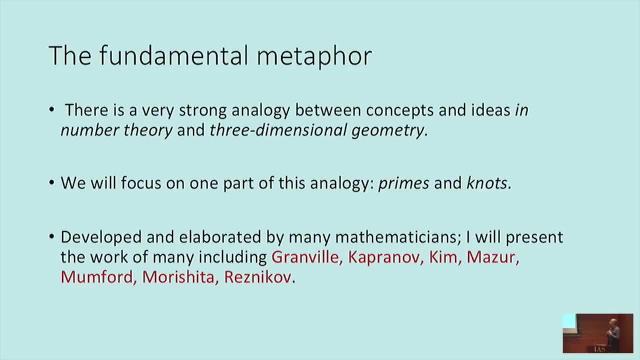 And this is So. this is something. It's not my work. It's something which has been developed and is developing by many mathematicians over the last half century, So I'm going to be talking about the work of many other people And, at the end, it's certainly very much. 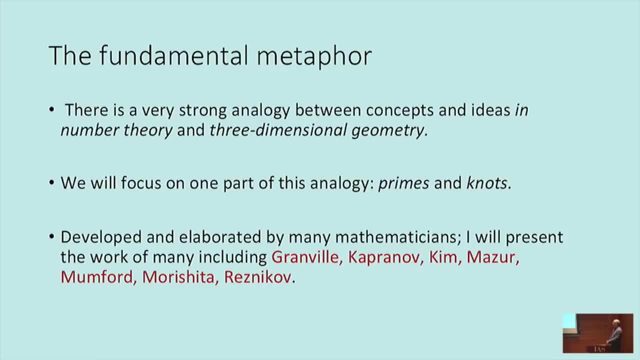 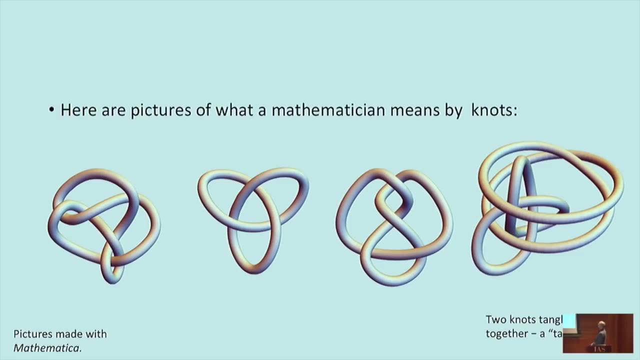 It's very much influenced the way I view things and I'll say a bit about how it influences current research in number theory. Okay, So we're going to start by talking on the side of knots. Okay, So, this is what a mathematician So I think informally, when you say knot, you can imagine taking a piece. 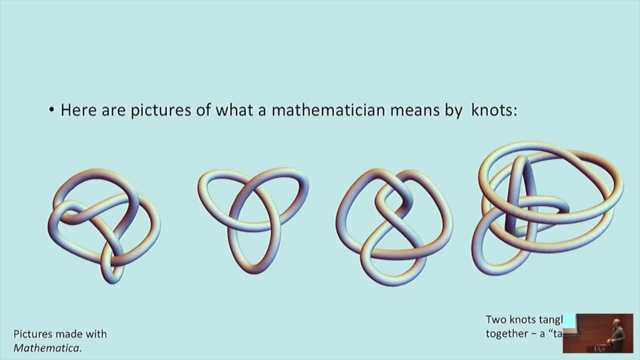 of rope and tying a knot in it. When a mathematician says knot, they always mean that the free, that the free ends should be tied together or closed up. Okay, So these are knots. There are no free ends. That's what, in math, the word knot refers to. On the right-hand side. 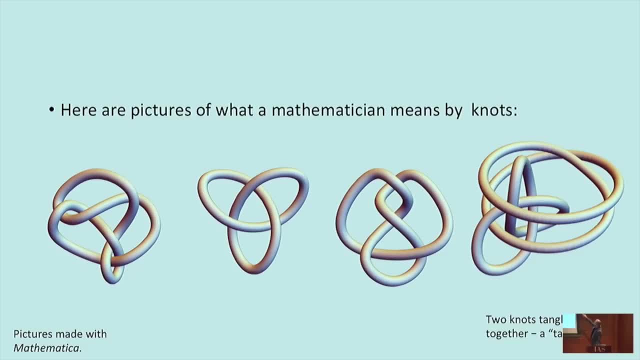 here you have something very slightly different. There's actually two knots here, So if you look carefully, there are two of them which wind around each other. Okay, So there are two loops winding around each other in a complicated way, So the mathematical term for that is link. 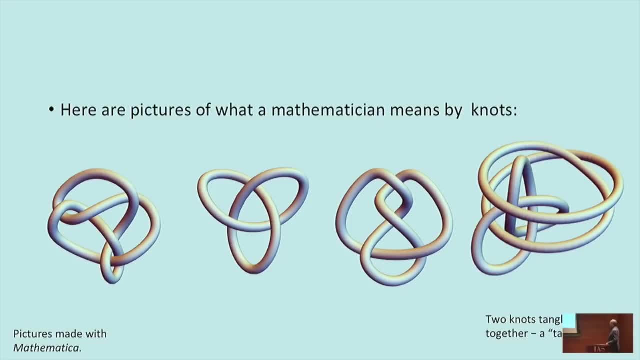 But for the purpose of this talk I'll use just a more informal word: tangle. Okay, So to study knots. we want to produce knots, which I think is usually not what one wants to do- the opposite most of the time- But I want to have some systematic way of producing. 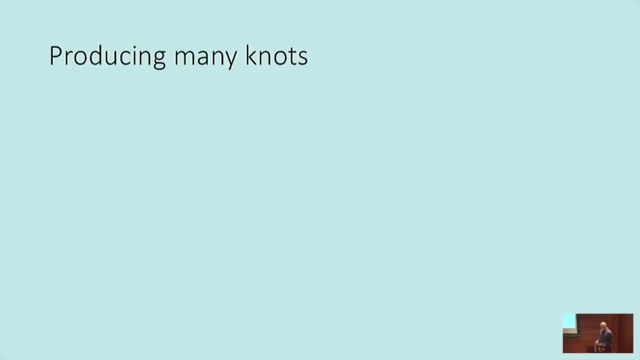 knots so we can talk about studying them. Okay, So before I show you, I'll just do this. When I wanted a prop for this talk- It's a shame this is live streamed- I went to my children's toy box and I stole some. 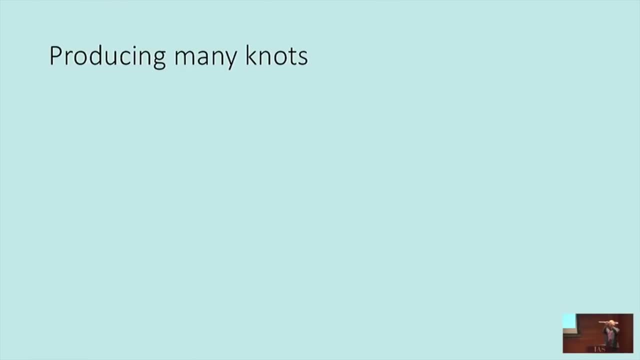 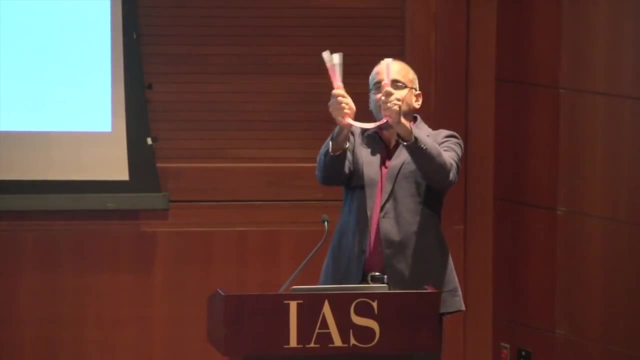 glow sticks. So these are you could. these are each sticks. they glow when you bend them and you can connect them up. Okay, So a simple way you can make a knot is you take a bunch of these and you connect them, but you sort of twist them as you do it. Okay, So maybe 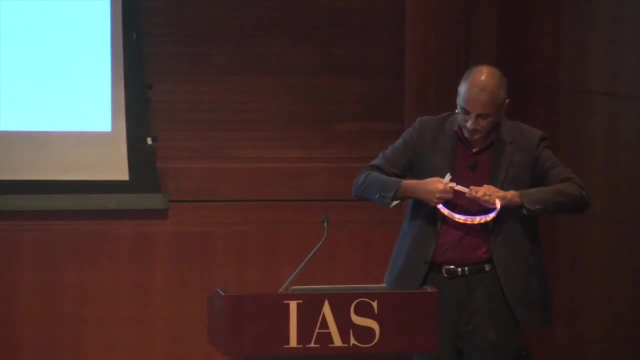 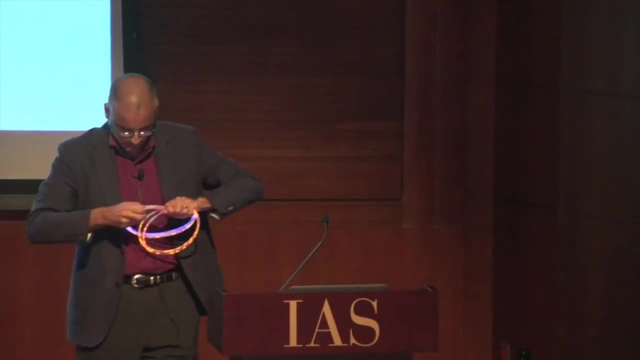 you could dim the lights a bit here so it will look nicer, All right, So once you connect the ends. so I took five glow sticks and I just connected the ends, but I twisted them along the way. Okay, And when you do that, what you get? 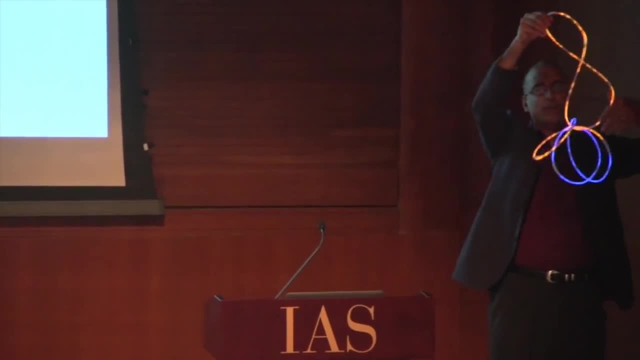 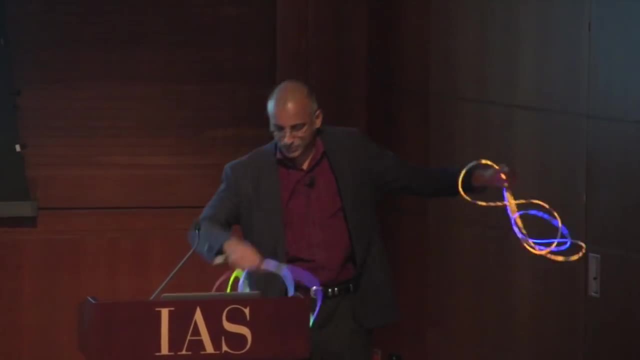 and I don't know how well you can see this, but they, they will form some number of linked knots. Okay, And because I wasn't really sure that would work out, I also did it a few times before. Okay, So, 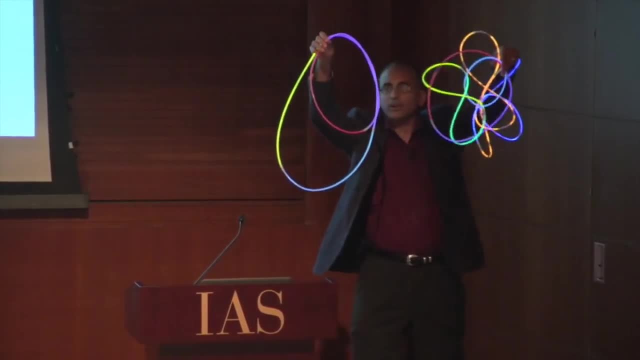 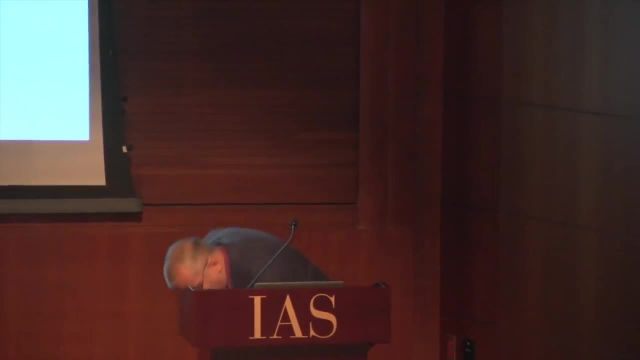 Okay, So Okay Now. the more the point is, the more you tangle them. Okay, Let's just leave the um. the more you tangle them- And here's one where I tangled a lot- the more complicated the 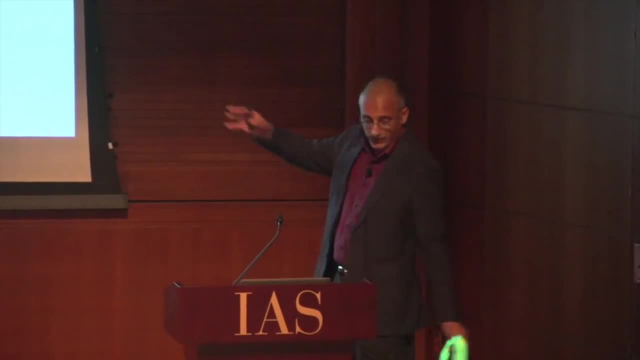 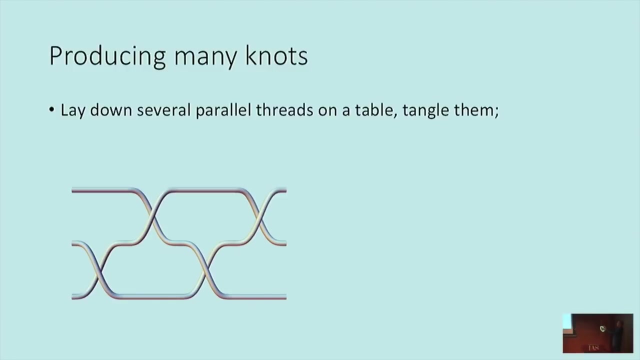 knotting gets Okay. So let let me just say what I just said, what I just did. I'll say it in words: Um so said in a uh. so, instead of glow sticks, imagine threads, Okay So. 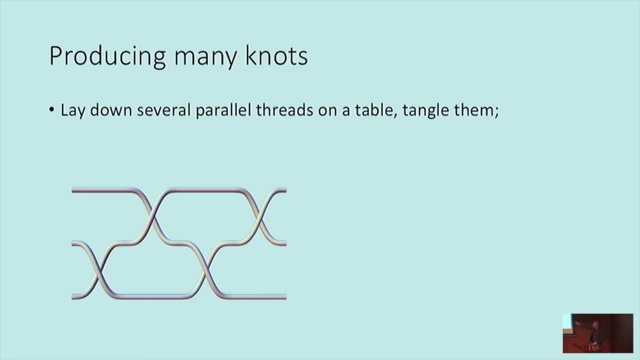 you lay them down on a table and you tangle them, which in this picture means they're connected. You cross them like this And then I bring the ends together. So I pick up the right-hand side, bring it to the left-hand side and join it. And if you look at what, 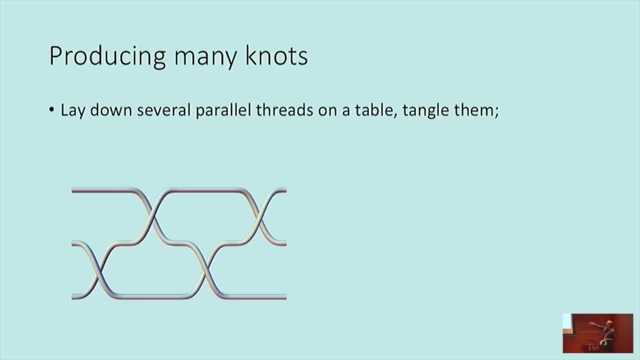 will happen. they will connect into one long thread and the picture it will- if I did it right- ends up looking like this: Okay, So this is a sort of systematic way we can produce knots. We take our threads, we we crossed them And, if you want, we can record. 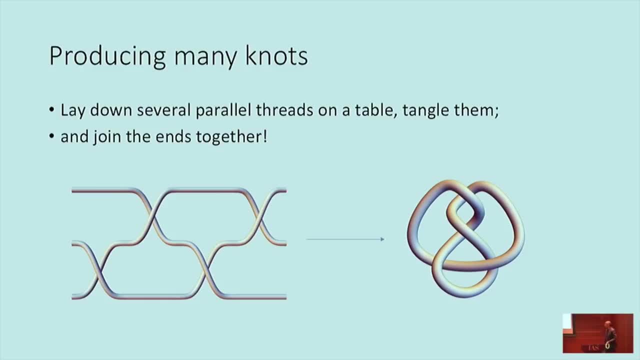 how we crossed them. We can repeat exactly the same thing again And we joined the ends together, All right. So imagine for a moment: you do this many, many times, like I did, and then you get this collection of- uh, a whole bunch of of knots. each time you do the tangling in a different 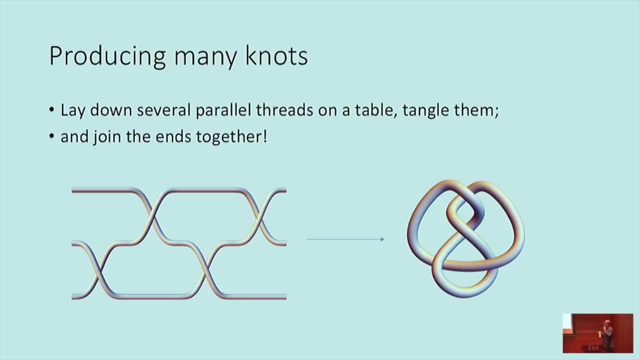 way, And so you have all these knots and you then wonder what we can do with them. Okay, So we'll come back to that, All right? So I'll just imagine your mind: You've you've done all this and they're lying on your desk and we want to at some point make some sense. 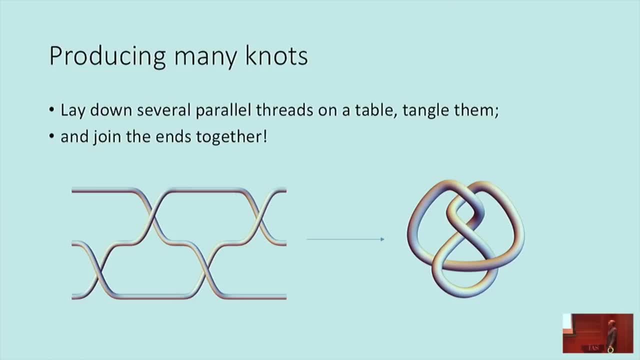 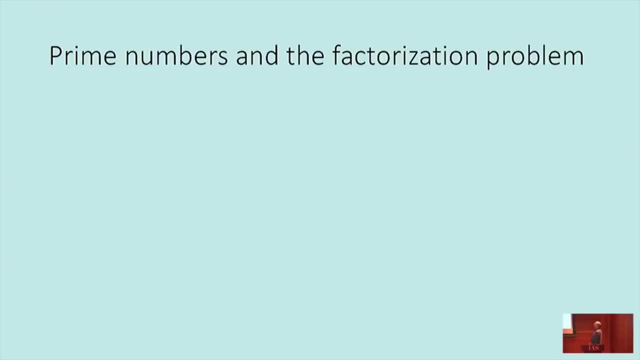 of it, but we'll. we'll come back to it in a moment. Just hold that in your mind. I now want to switch to the other side of this talk, which is the side of numbers. Okay, So I hope many of you will have seen the notion of prime number before. A prime number is a whole number. 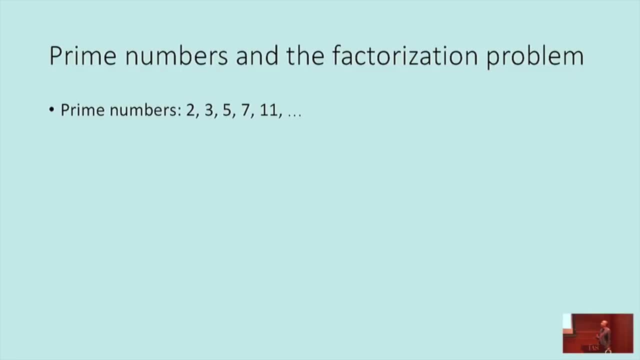 So, Okay, It is not the product of two smaller numbers. So, for example, six is not prime because it's two times three, but two and three and 13 and 19 are all prime numbers. Okay, Now, if you go to a undergraduate course on number theory, I think there are two, there are two. 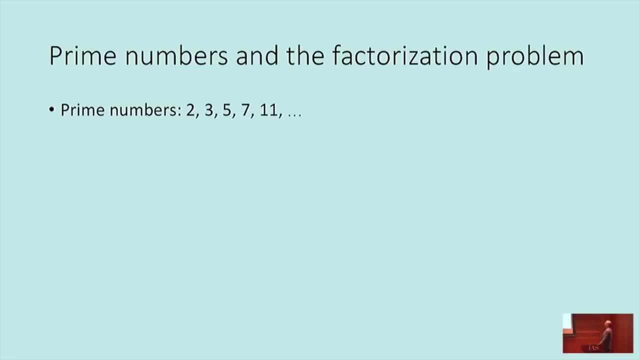 very important things you'll learn in the course, And we're we're going to touch on both of them in the talk today. But the first one is that every number is a product of a product of prime numbers. Okay, So, for example, a thousand and one is seven times 11 times. 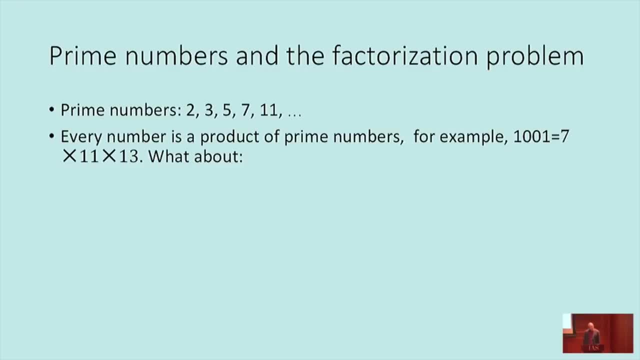 13.. Now, there's only one way: that it's a product of prime numbers. Okay, Now, if you make that number much, if you take a bigger number, okay. so here's a number with, I think, uh, 50 digits. Um, we still know that it is a product of prime numbers, but it's not so. 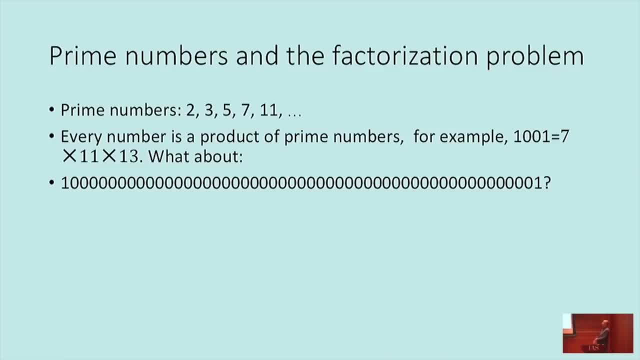 simple, So to find out what they are. and I think a hundred years ago there would be no way that anyone could have written this as a product of prime numbers. Okay, Now it's a matter of a second on a laptop. I will tell you that this, that number up there, is this product. 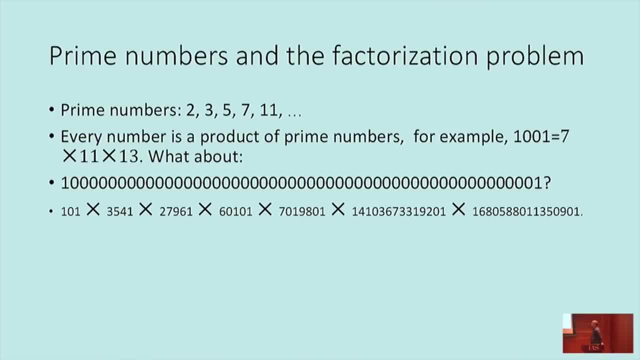 of prime numbers. Okay, But this is- uh, it's still so. it's quite difficult to do. So if I make this not a 50 digit number but a 500 digit number, very likely that there's no computer today. 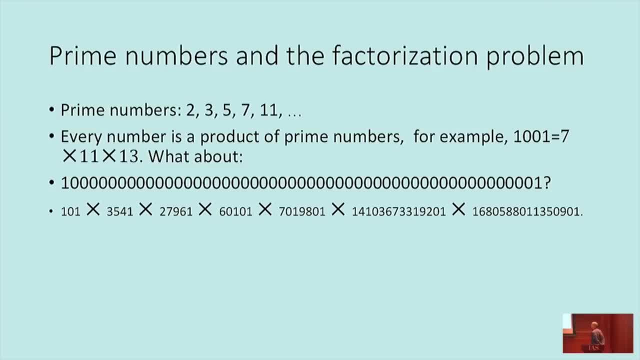 And that could factor it into primes. Okay, So this is it's. uh. now let me just say one direction of this is easy, Like if I give you this, all these prime numbers, you can multiply them together and check that they give that. it might take a while but you could. 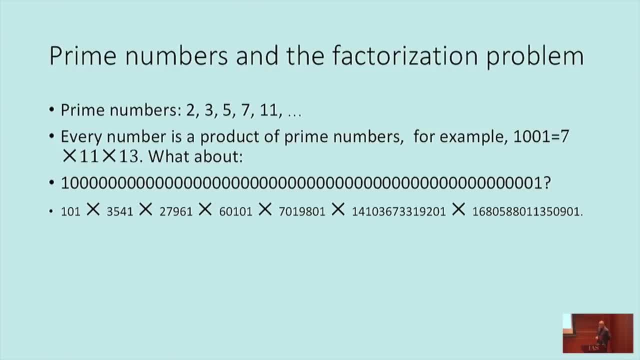 might take. you don't want to do it, but you could- But, on the other hand, going the other way, that is, if you start with a number and you need to produce the primes. that is, if, as I said, if the number is very large, that's fine. But if you start with a number and you 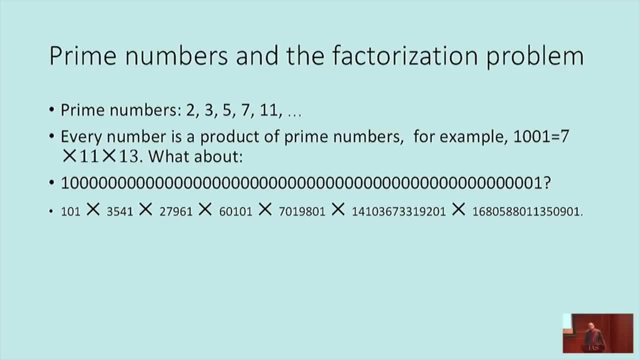 need to produce the primes. that is, if, as I said, if the number is very large, that's fine. It's not hard, That's becomes extremely difficult, even with a super computer. So if you have a problem like that, that's sort of easy to do in one direction. it's easy to multiply prime numbers. 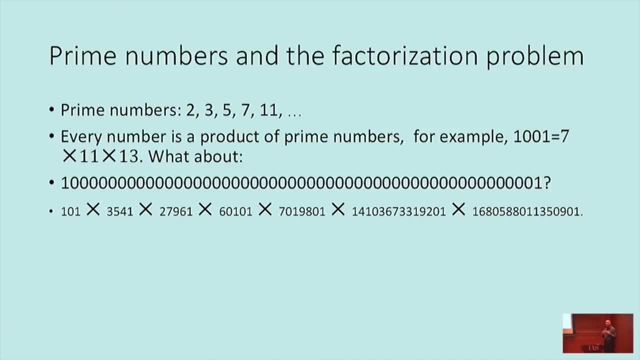 but difficult to go in the reverse direction. it often can be used as the basis for a crypto system. Okay Now, the talk today is not about um cryptology, but I just want to mention this, uh, that the fact that factorization is. 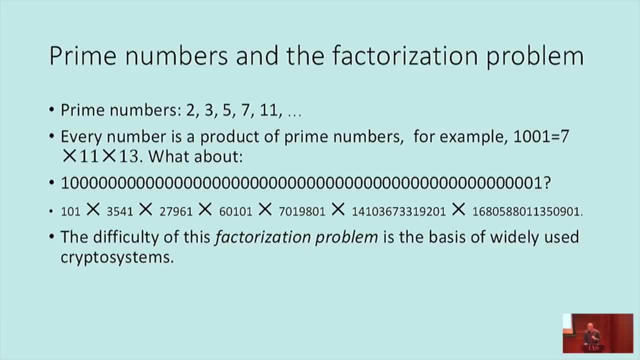 Ah W a difficult problem And sorry, maybe I didn't say it. By factorization I mean this question of given: if I give you a number, you have to tell me which primes it is a product of. So the fact that that's a difficult problem is the basis of some of the most widely used 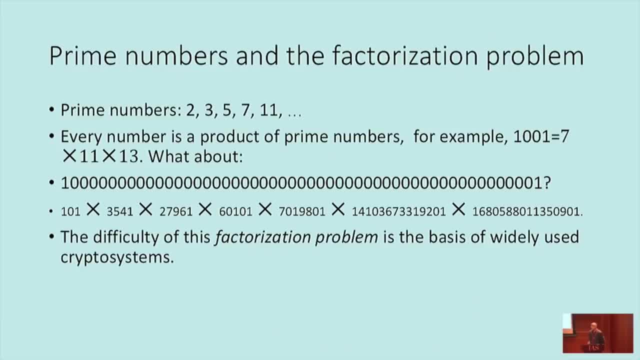 crypto systems Okay. so they're very broadly used in internet communications, And one of the reasons that the development of a fully functional quantum computer would be so significant is that it would be able to easily break this factorization problem, And that would require 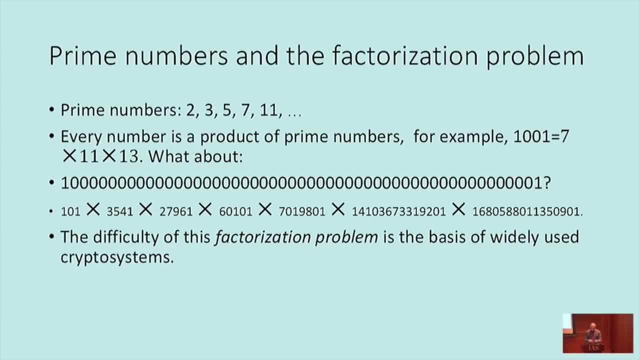 a huge rethinking of how one designs crypto systems. Anyway, this talk is not about that, but I wanted to mention- we're going to talk a lot about factorization, so I wanted to mention what its technological context was. Okay, so I'm going to, if I 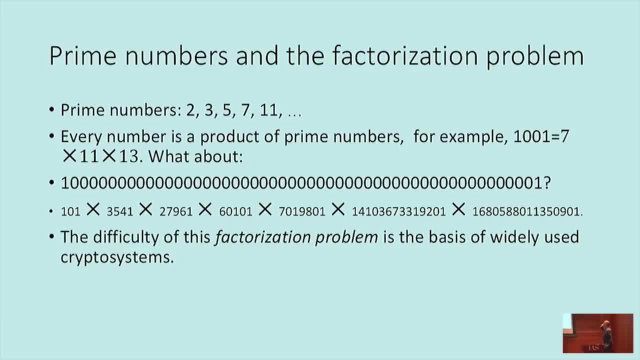 All right. so I gave you one number and its factorization And you'll notice that, relative to the number of digits in the original number, all the factors were fairly small. Okay, they have relatively few digits And if you keep fact you can wonder how typical that is. 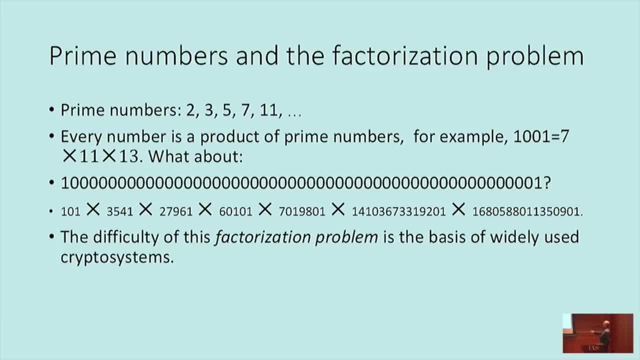 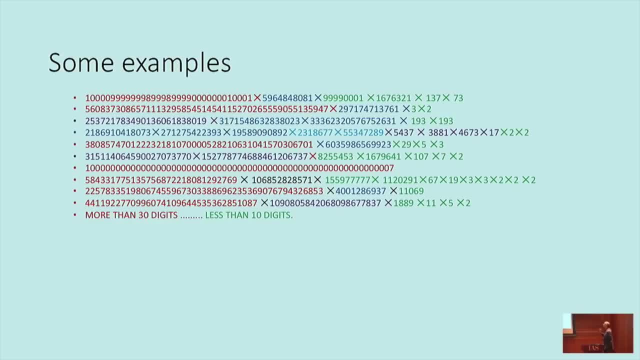 Okay. so let me give you the factorization of some more numbers and we'll Okay. so this Here: what I did is I factored 10 60-digit numbers. Okay, they don't look like they all have the same length, but that's because of the way the formatting works. They were all 60 digits to start with. 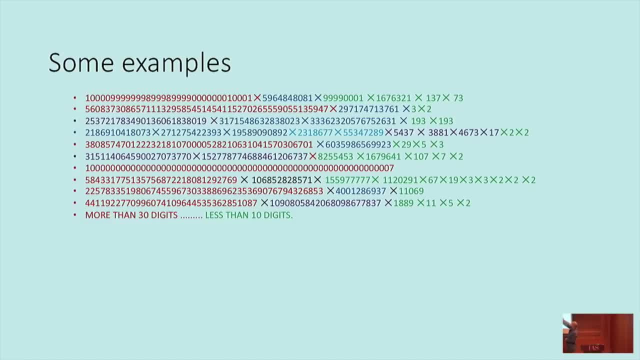 And I'm sorry I think these colors don't come out very clearly, but I color-coded it, So each one, each line of this is a 60-digit number written as a product of primes. The red are the largest, are large primes. 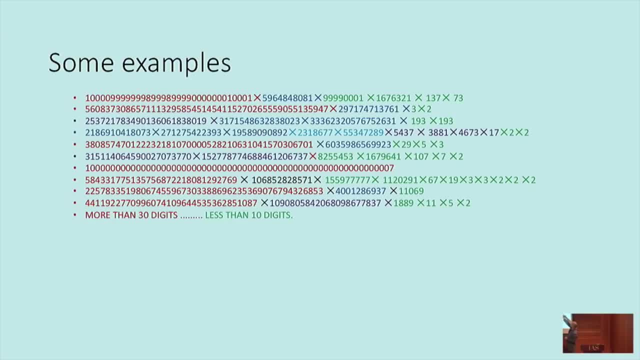 So that's more than 30 digits. Green is less than 10 digits. And then there are some blue intermediate colors for intermediate number of digits. Okay, so I'm not, You're not meant to, Nothing is meant to jump out at you from this, except to say there's a fair amount of variation in what you see. 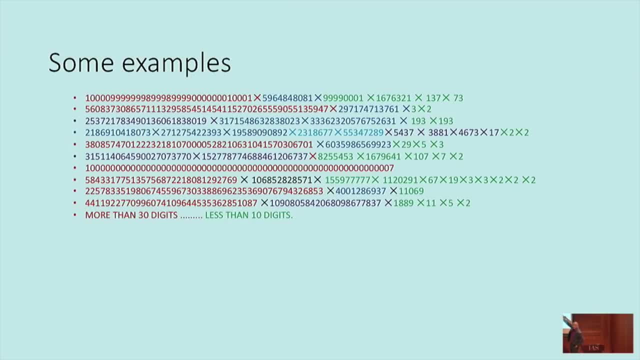 Okay, on one line you see 1,, 0,, 0,, 0,, 0,, 0, 0, and 7 at the end, And that's a prime number, Okay, so among these 10 numbers, one was actually prime. 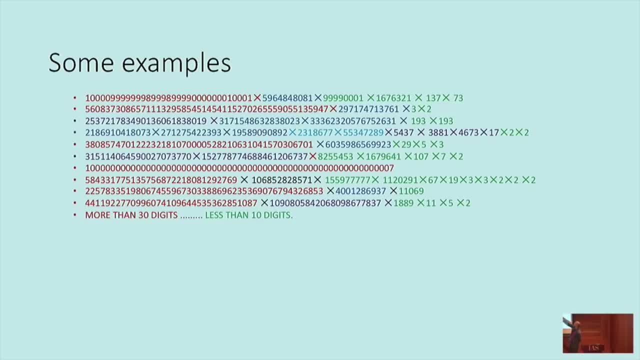 Some numbers, as the one on the previous slide, have only fairly small factors. Maybe the only thing you notice is most of them have a fairly large factor. Most of them have a factor in red. Okay, and fairly large here means a prime with more than 30 digits. 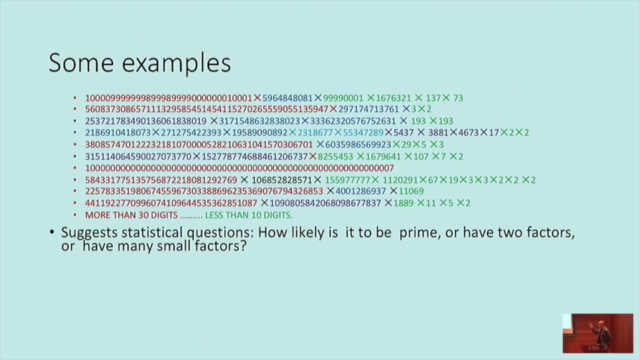 Okay. so if you start looking at this, you see it's very It's quite irregular what happens. Okay, so if you start looking at this, you see it's very It's quite irregular what happens. And you wonder how often is a number prime? Okay, if I write, If you write down for me a 60-digit number, you just write 3,, 4,, 9,. you keep writing at random 60 digits. 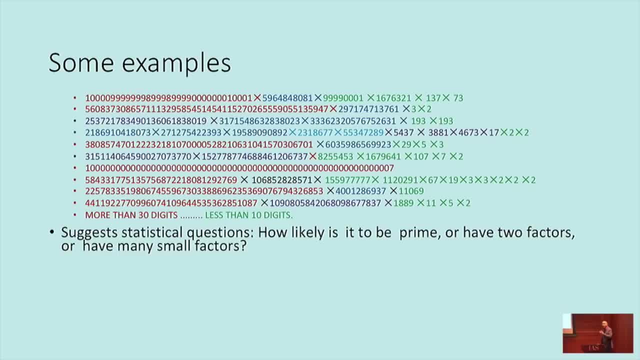 how likely is that to be prime, or have two factors or Okay? so you can keep asking many questions like that And these It's essential, It's not just a matter of curiosity. This one, the understanding of the, The factorization of typical numbers, is very important in practical cryptography. 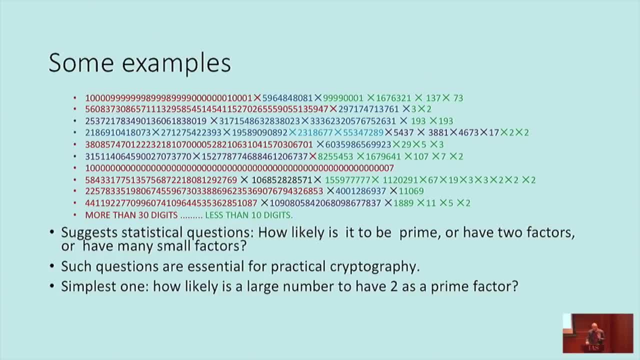 Okay, so So I'm going to tell you on the next slide, I will tell you So, these type of questions about how likely is something, the factorization, to look a certain way, Although we can answer them, and I'll tell you some of the answers on the next slide, okay. 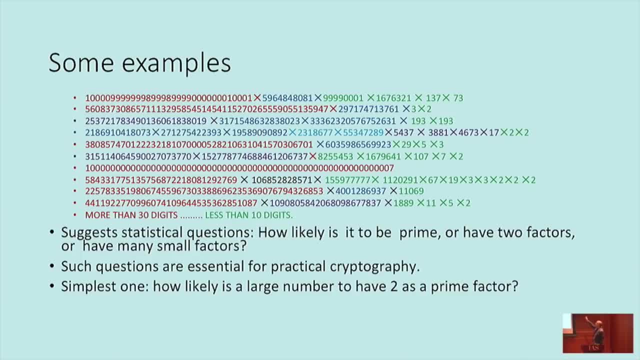 Although we can answer them, and I'll tell you some of the answers on the next slide. okay, I'll tell you how we got them And, in lieu of that, let me just talk you through a very simple example before I give you the more complicated answer. 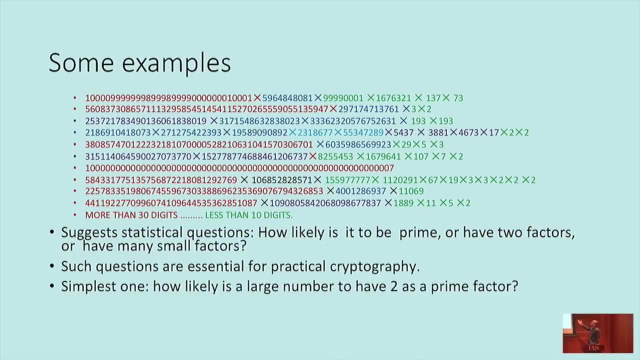 So the simplest question you can ask about factorization is not really: is a number a prime? The simplest thing you can ask is: is 2 one of its prime factors? And so a number has 2 as a prime factor if it's 2 times something. 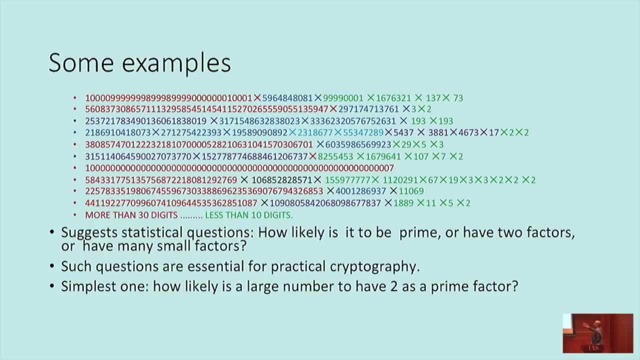 So if it's an even number and every second number is even so, the likelihood of this is 50%. So that's very simple. But all the answers I give on the next slide are kind of reasoning at the same level but in a much more complicated way. 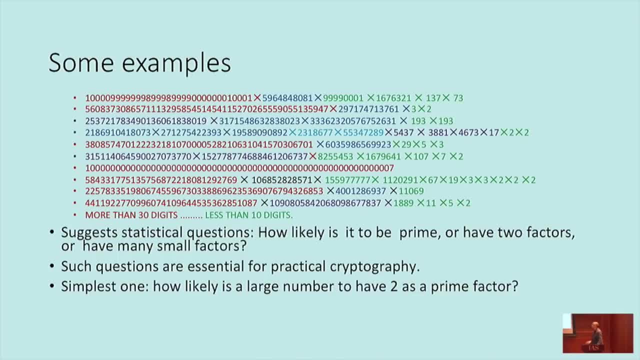 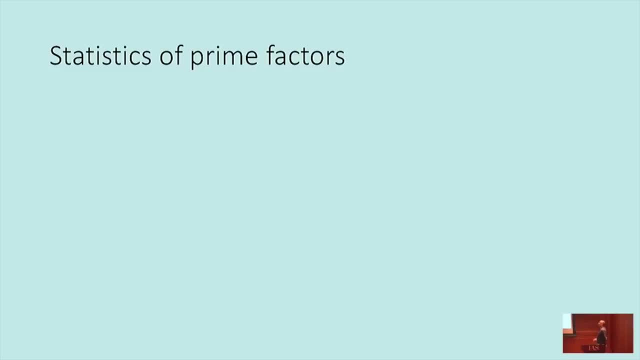 Okay, so this simple question gives you a sense of how you might go about. All right, So now I'm going to give you a table of some of these statistics, And the exact answers aren't important. Okay, so you don't need to focus on what the numbers are. 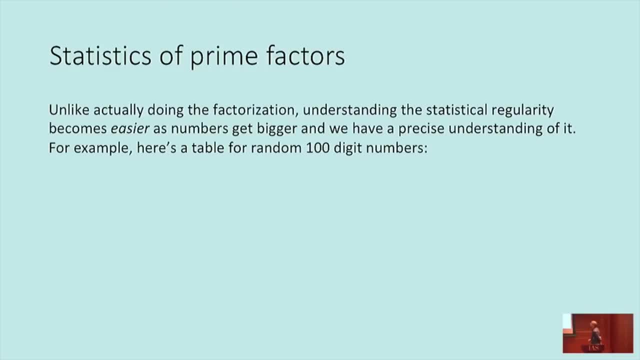 The main point I want to make, which I'll say before the table, is that it's very hard to factor, as I said, a 500-digit number. However, we actually have a very good theoretical understanding of the statistics of how it factors. 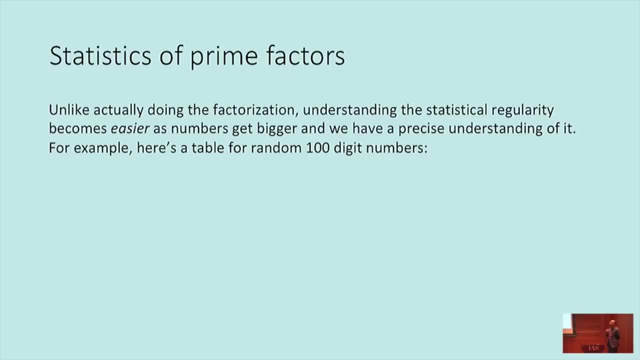 So, even though it's harder to actually factor it, our understanding of how likely it is to factor a certain number, how likely it is to factor a certain way, becomes better and better as the numbers get larger and larger. Okay, which is maybe a little counterintuitive. 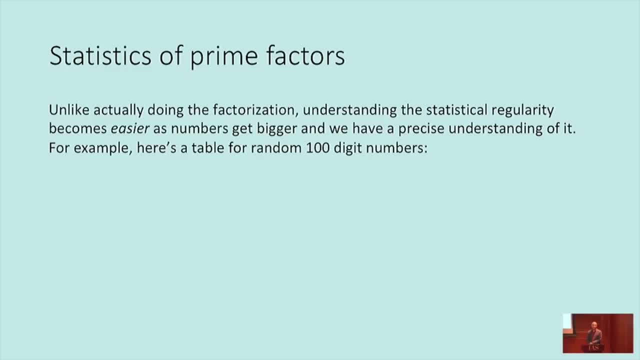 but so this sort of statistical questions become easier as the numbers become larger. So, even though you can't simulate it, nonetheless we can understand it. So here is, I'm going to give you a table which tells you about 100-digit numbers. 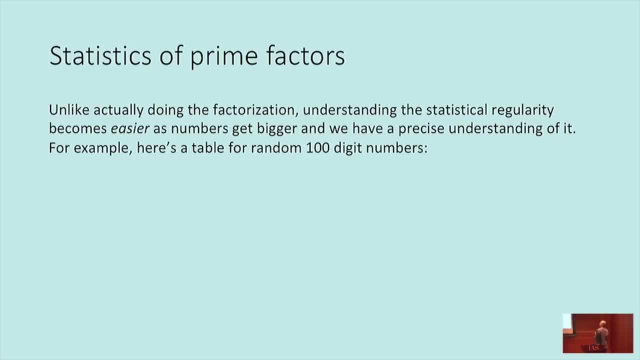 So if you gave me a 100-digit number at random how likely various options for its factorizations are, Okay. Again, the exact numbers aren't important, Okay, I'm just giving you this as examples of the type of thing you might ask. 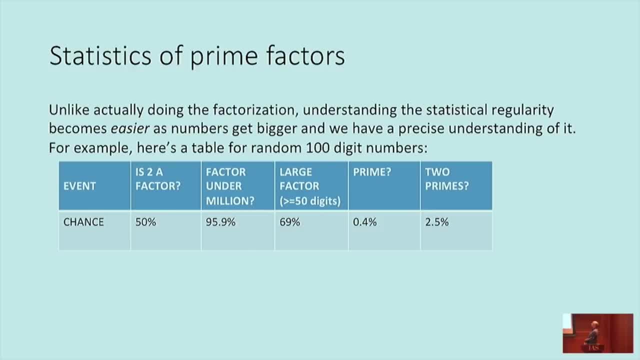 And so we discussed the first one. How likely is 2 to be a factor? It's 50%. How likely is it to have a prime factor which is less than a million? All right, and that turns out to be about 96%. 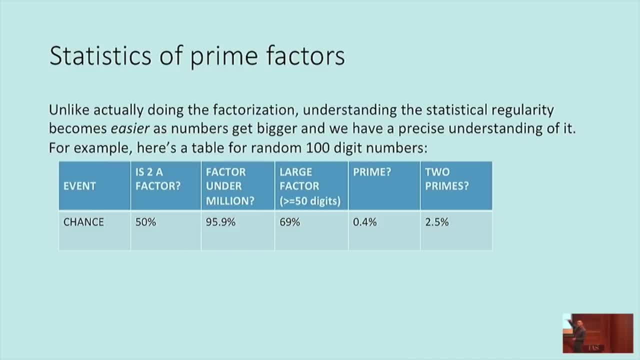 This middle column is the analog of that of the numbers which had red factors in the table before. These are the numbers that have a prime factor with 50 or more digits- about 69%, And the chance of actually being prime is about 0.4%. 1 in 230. 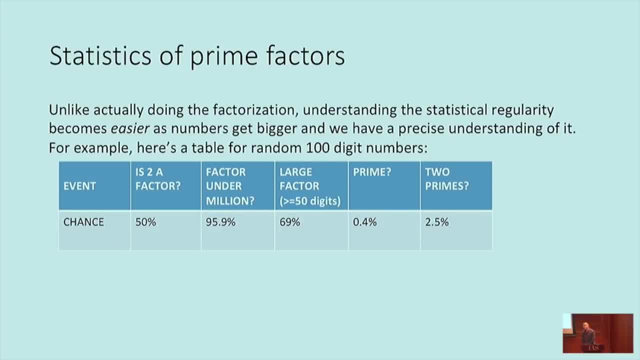 Okay. so it's quite rare for a 100-digit number to be prime. It's a little more common for it to have exactly two prime factors. Okay. so I could go on, but I restrain myself, And now we've reached this point. 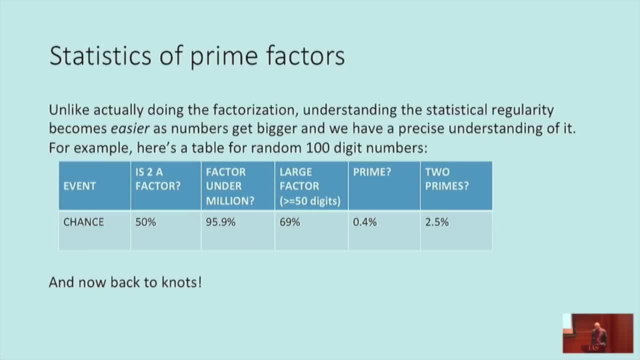 We will go back to knots. So where I left knots is that we went and produced all these knots- I'll remind you of that in a second- And I didn't say what we would do with them And what we're going to do with them. 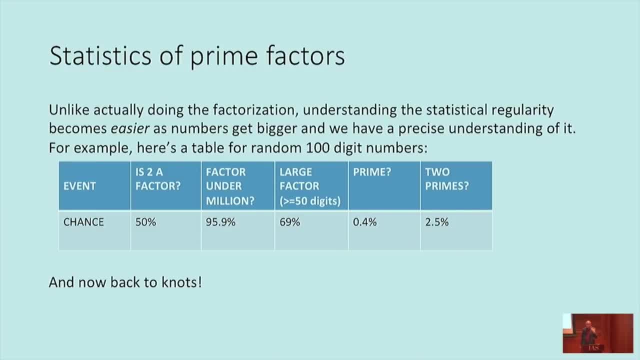 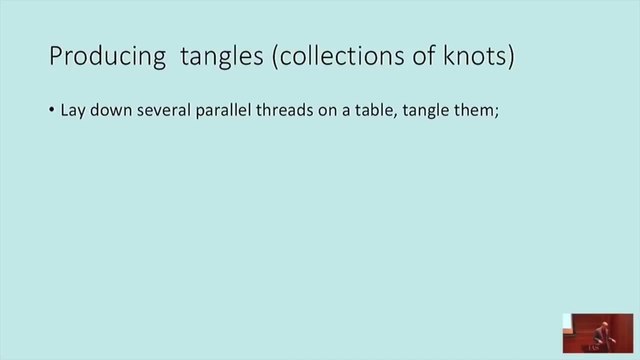 is. we are also going to consider some, we're going to do statistics on them And we'll see that the answers are the same as what we found in this table. Okay, so I'm just repeating now what I said before. Okay, we have this process for. 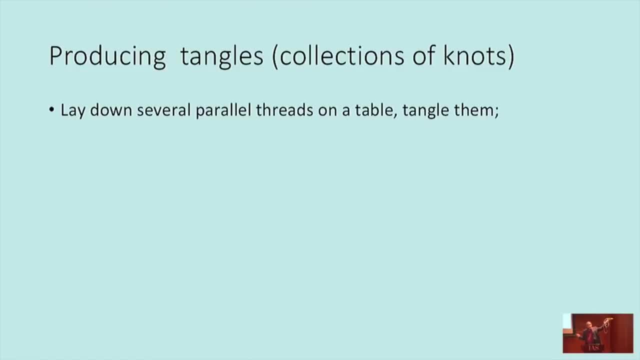 you lay down a bunch of threads and you know you join them and you get a knot. You do it again and, depending on how you do the tangling, you get a different knot. Okay, and now I have to say: 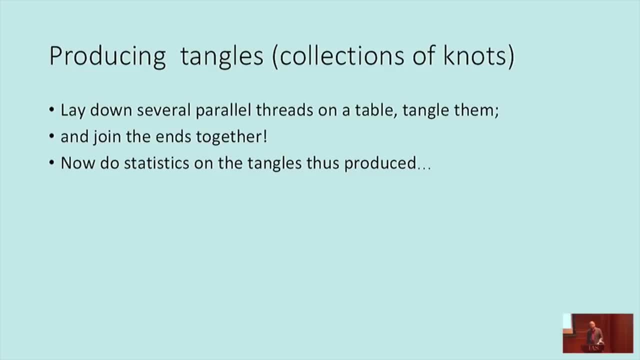 you know, to get to the point where we can do interesting statistics, you can't just use five threads or five glow sticks, you have to use hundreds. So this is, you know, physically unrealistic. but it's very easy to simulate this on a computer. 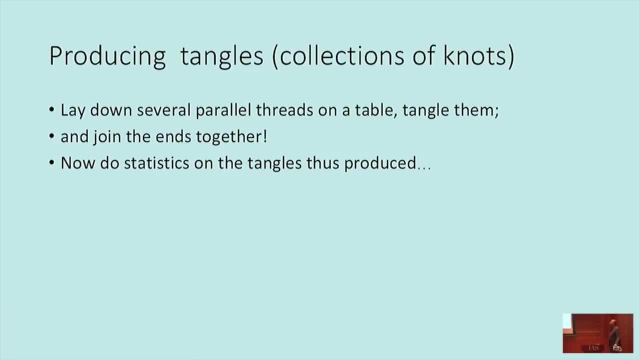 Okay so this model is sort of a little bit misleading. Okay so here's a kind of pictorial representation of this And I want to draw your attention just to a couple of features. So remember, here I took five glow sticks. 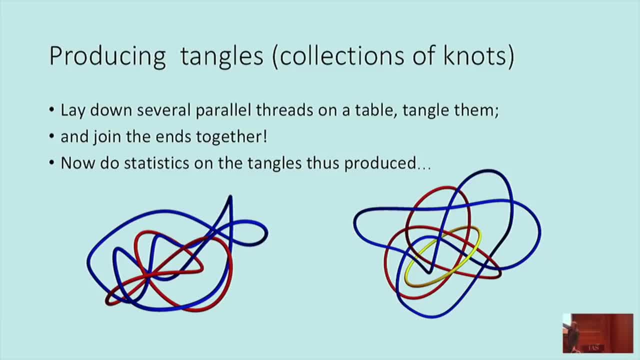 twisted them, joined them and I get in general, some collection of knots which are tangled together. Okay, it may be that all the five glow sticks stay, for example, okay, well, what is this here? You can't really see this very well. 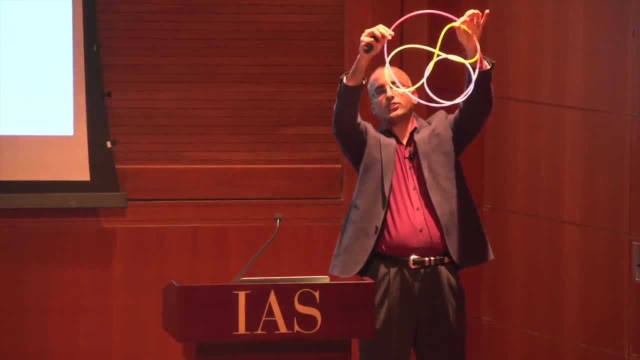 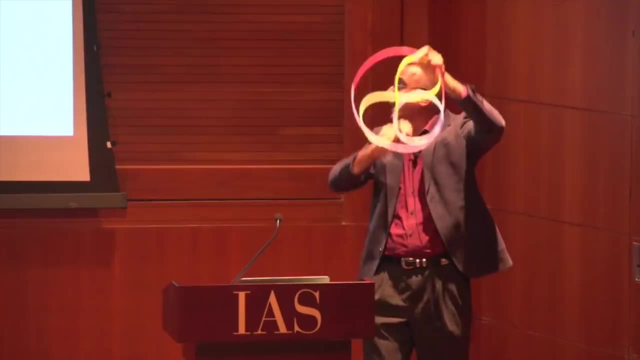 but I started off with five glow sticks and what you get is two knots each involving two of them and one that involves one of them. So those five have split into two plus two plus one. So, in general, when you do this, 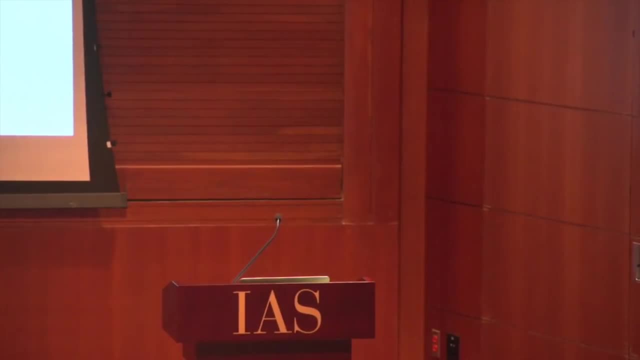 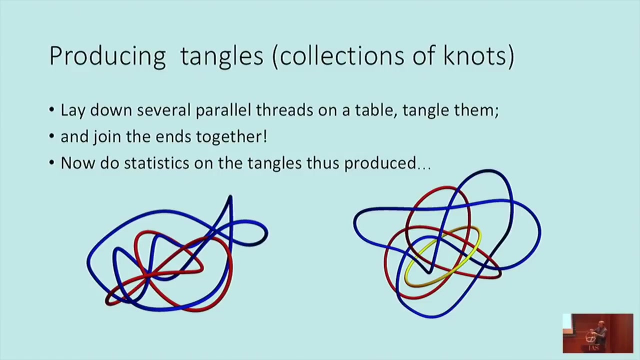 you will get some number of knots that are tangled together. The number of knots may vary and the length of the knots will vary. Okay, because different numbers of these glow sticks merge into knots. So on the left you have two knots. 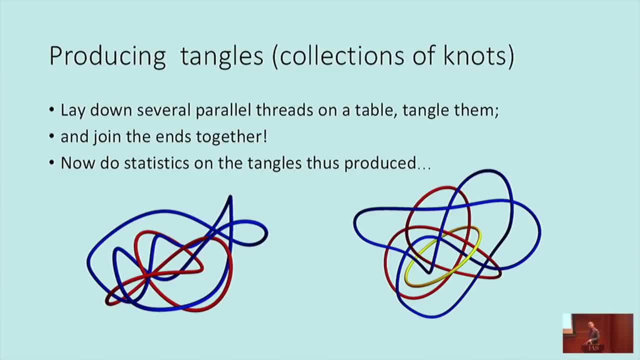 on the right you have three, and again the lengths will be different. Now, what's kind of most interesting about this is how the piece is tangled together, But we're going to come back to that issue. Okay, we're going to ignore how they're tangled together. 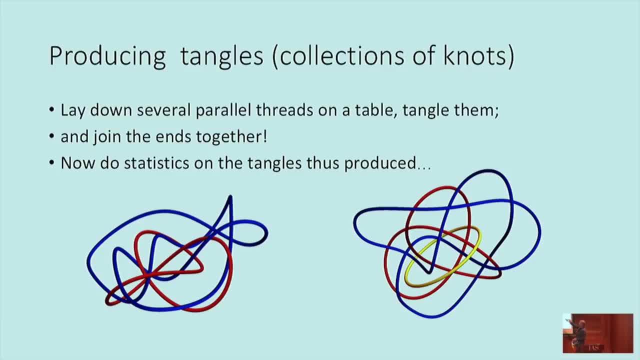 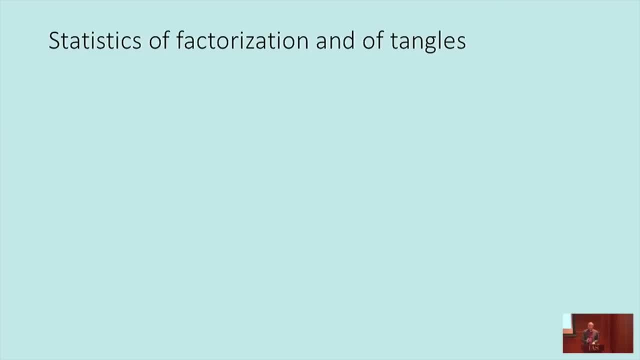 and just ask about how long they are and how many of them there are, And we'll compare that to the statistics of factorization. So what I'm going to do is that table. I gave you a table of statistics of how you factor a 100-digit number. 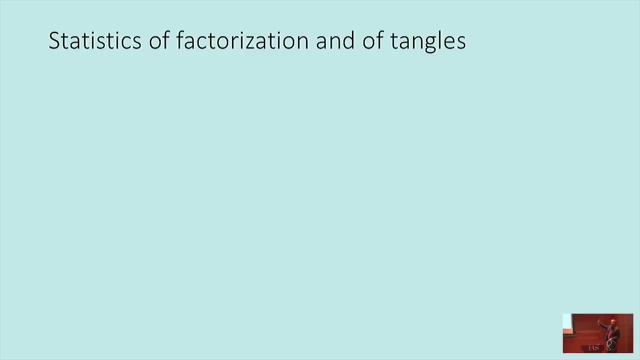 and one by one. one by one, we'll go over the. For each question, there'll be an analogous question about this and, after some work, all the questions except one will have an analogous answer. Okay, so the simplest question to discuss is: 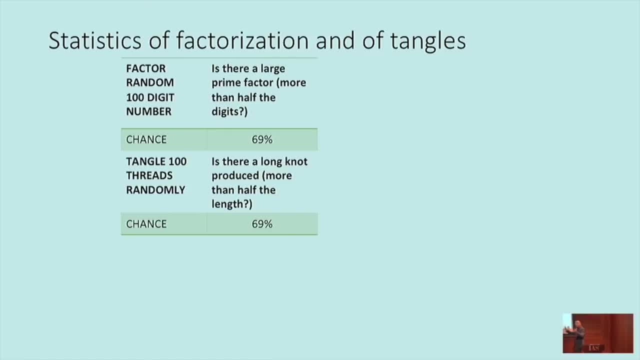 When I factored a 100-digit number, I said the chance that it has a large prime factor, which means more than 50 digits, was about 69%. Now suppose I do, And, by the way, I maybe should emphasize this. 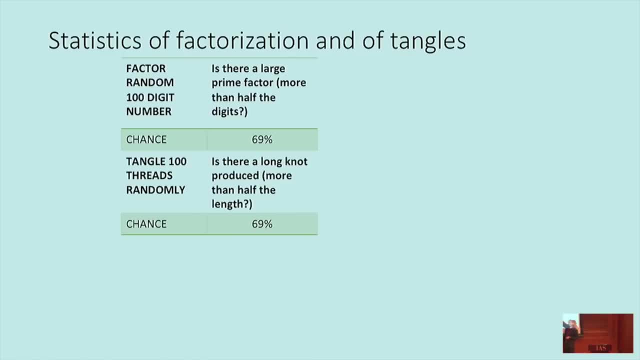 The answers to these type of questions will change when you change the number of digits. Okay, this will be one answer for 100 and different for 1,000.. So suppose I do the same thing with my knots, except starting with five threads, as I did here. 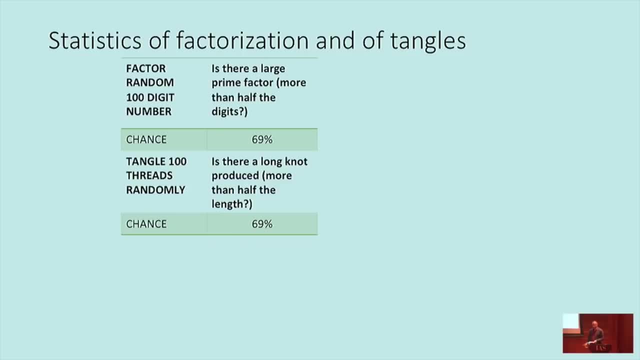 I start with 100, okay, I started with a 100-digit number, so I'll try 100 threads And I ask: among all the knots produced, is there a long one? And I define long as, analogously, It's more than half. 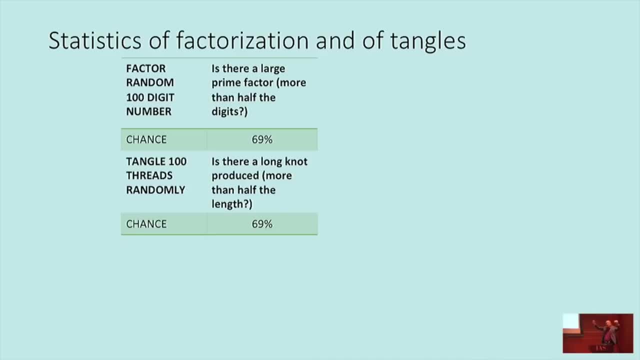 It involves more than half of the original thread. So if I had 100 threads to start with, do I produce a knot that involves more than 50 of them? And you can easily find by simulating or theoretically. the answer to that is also about 69%. 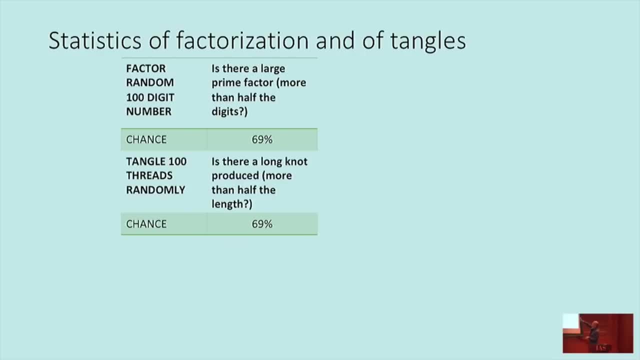 Okay, so what we're gonna do. These questions are analogous and the analogy will be: primes are like knots, so the word prime will be replaced by knot and the number of digits will be replaced by the length of the knot. okay, 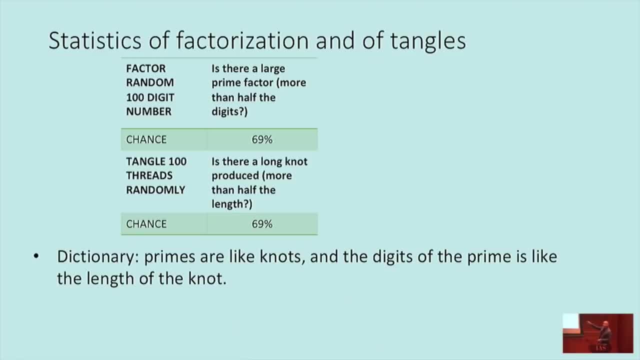 So the next. Now I'm gonna add two more entries, okay. So in my original table I had asked what is the chance of one prime factor, which was about 0.4% If you And the analog of that, all right. 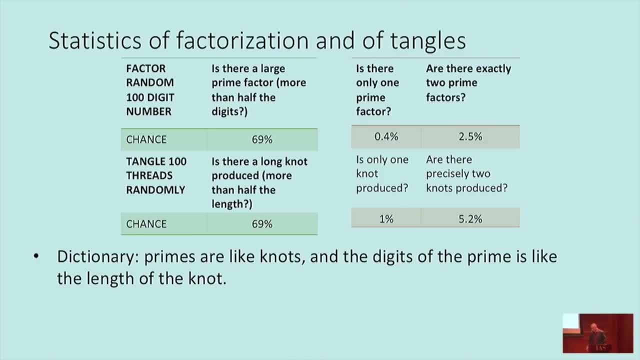 The analog When I make my tangle. the analog of having just one prime factor is that you just get one knot. okay, That is all the five threads, or 100 in this case, joined into one long knot, It turns out the answer to that is 1%. 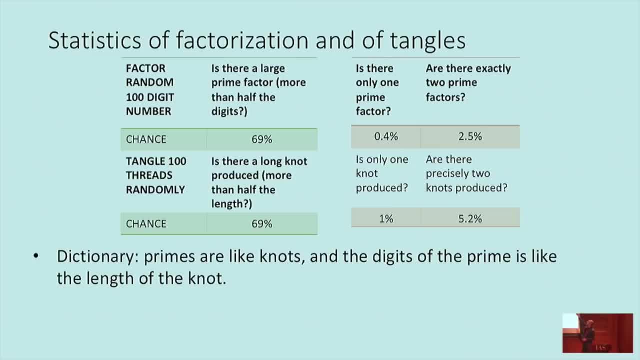 So it does not match with that, and similarly, other questions of the same nature will not match. So the problem here is that I sort of assumed that the 100 digits is the equivalent of tangling 100 threads. okay, And it turns out that there's a kind of exchange rate. 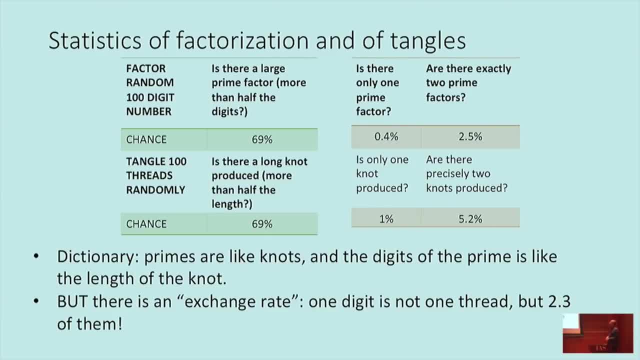 between those things where one digit is not really worth exactly one glow stick. It's worth 2.3 of them. So the analog of factoring a 100-digit number is doing this process with 230 threads. All right, so once you do that, 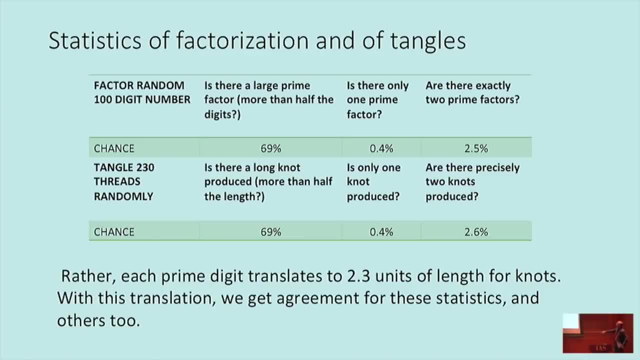 what you find is that these statistics match almost perfectly. There's a slight discrepancy in the last column, but all the All these slight discrepancies actually iron out when you go to larger numbers and longer knots. Okay, so I did 100 digits. 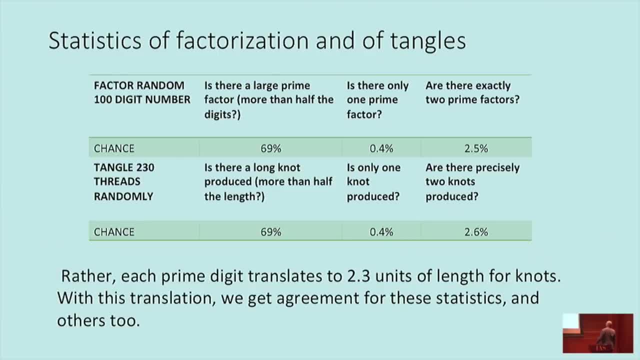 You could have made 1,000 and All right, there were two more entries in my original table and I will add those in now, because So I needed to first establish this exchange rate, which you could do experimentally, okay. 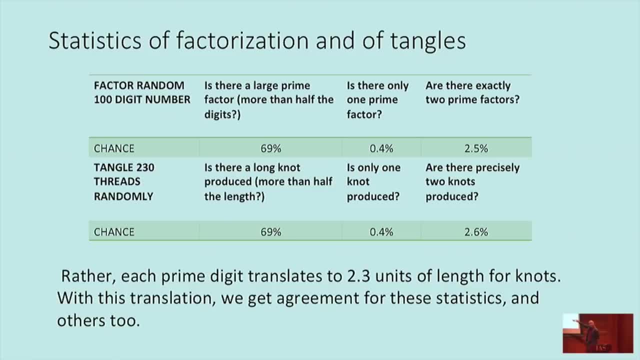 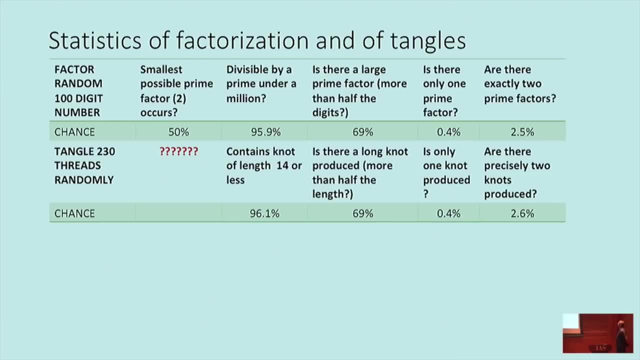 You could sort of try to match up one of the columns to fix this exchange rate, and then you would find all the others fall in place as well. Okay, so there were two other columns in my original table of statistics. The first was: 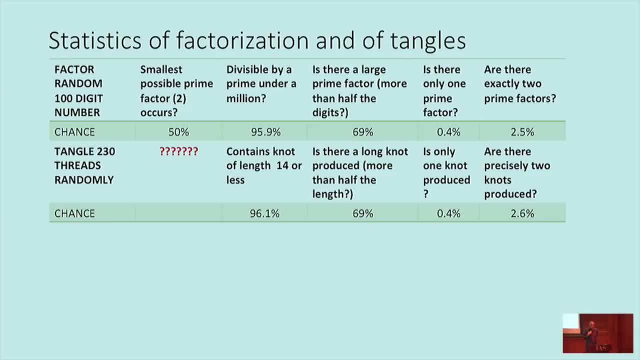 is it divisible by a prime under a million, That is, a prime with six or less digits. Now that I've established the, what the the corresponding notion for knots is. six digits corresponds to. So six times 2.3, it corresponds to something of length, 14.. 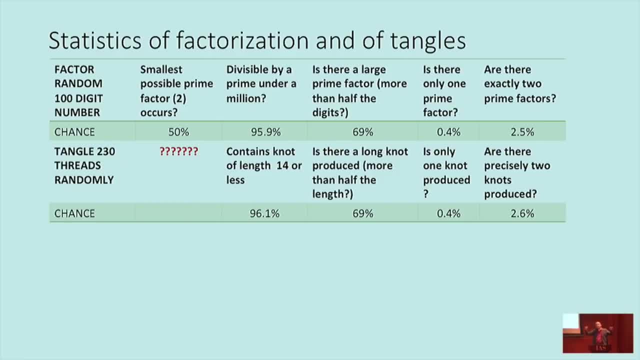 Okay, that is a knot that involves 14 or less of the original threads that you did took in this process And the chance of that is about 96.1%. So it matches very well. and again, as you go to bigger numbers, 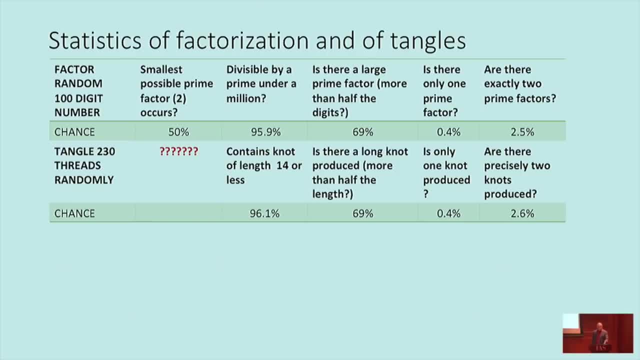 it'll iron out Strangely, the simplest thing you could ask, which is this question: does it? Is 2? a prime factor Does not have a good analog. Okay, so one might say that the analog 2 is the smallest prime. 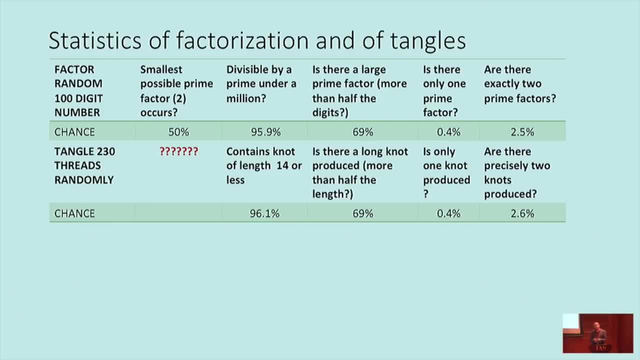 Perhaps the One should think of the smallest knot, which would just be a single glow stick, a single thread in a loop. That would not happen. That doesn't happen 50% of the time, It's more like 63%, And in fact there's just no reasonable analog. 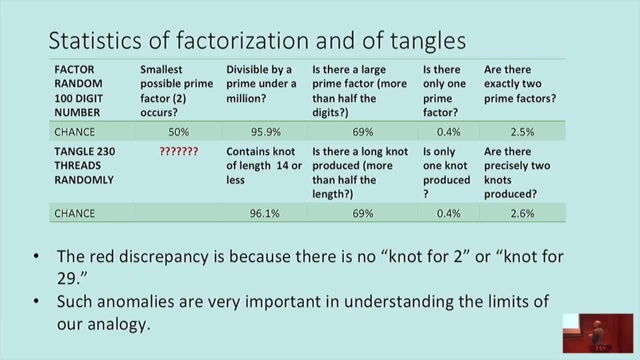 of that that we know. Okay, and this is an important point and I'm going to emphasize it before I go further. I mean, it's very. These sort of anomalies are very important in understanding the limits of this. So I say there's an analogy between primes and knots. 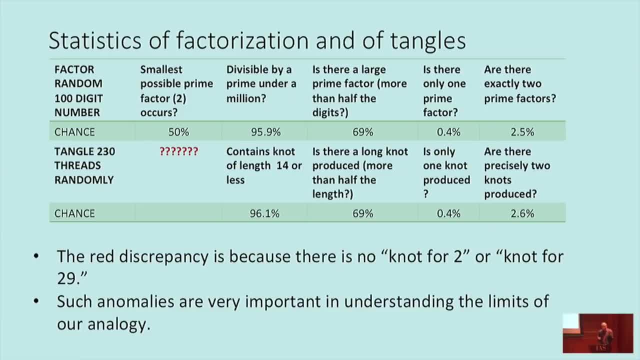 but this is not an. I'm not saying that for a given prime, there's no knot for 2, and if you For this knot, there's no prime for that. So it's more like the two things are governed by the same set of laws. 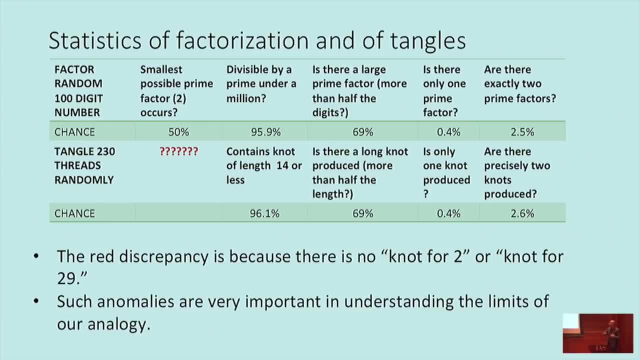 but it's not that you can go from one to the other or back. So there's no, There's really- We just don't know- any reasonable analog of that first question there. Okay, and that's because this analogy just breaks down at the level of individual things. 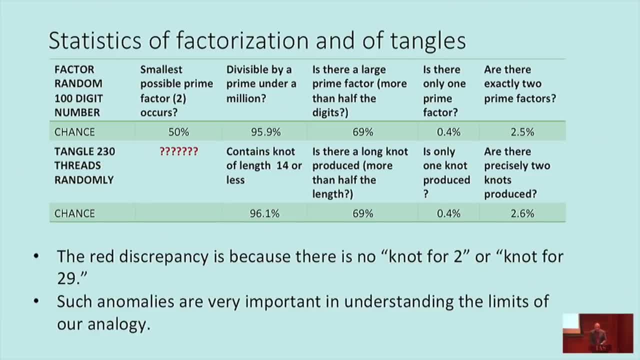 There's some sort of Correspondence of the underlying laws, as I said. but Okay, so that is. That's all for statistics. I now want to move. Go back to the. So, as I said, when you look at one of these knots, 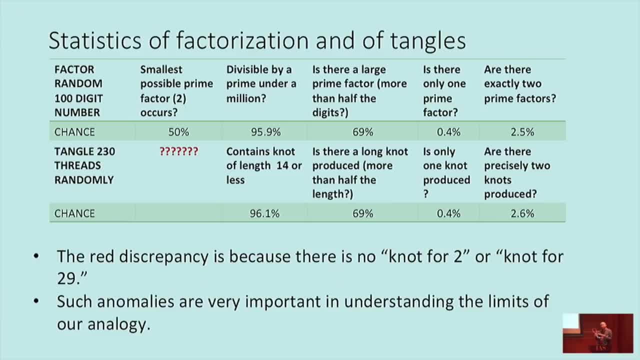 when I All the statistics I did, do not take account of how the pieces tangle together, And that's really the interesting feature of knots. okay, how they're tangled, not just how long they are and how many, but how they're tangled. 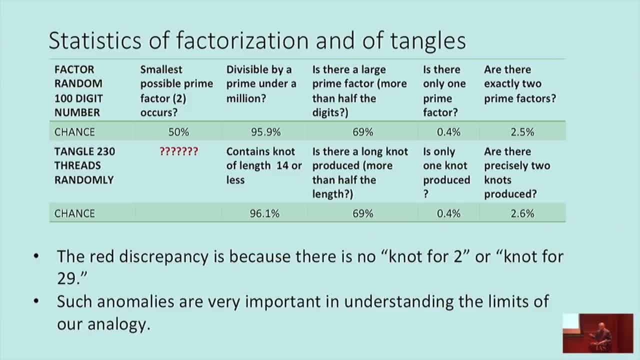 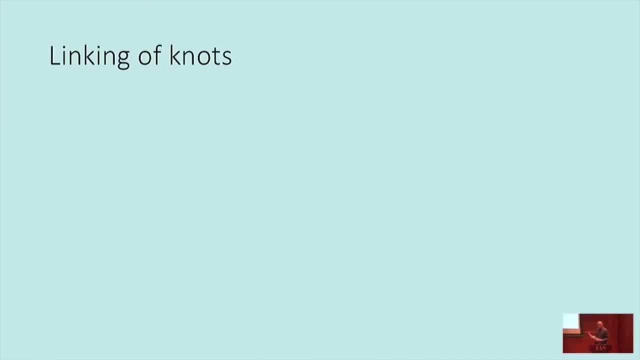 So I'm going to sort of I will now tell you a little bit of how that goes through this analogy. So the simplest This is a. At this point it becomes a huge story. but there's one very Suppose. I have two knots. 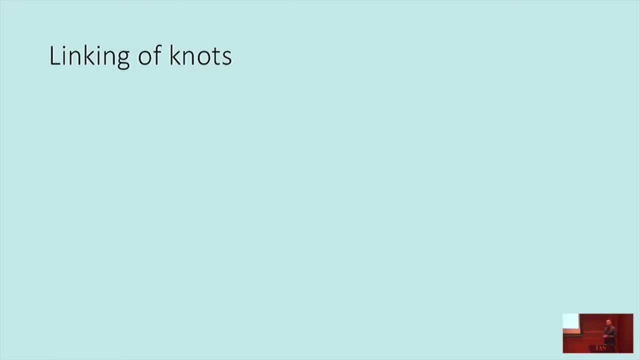 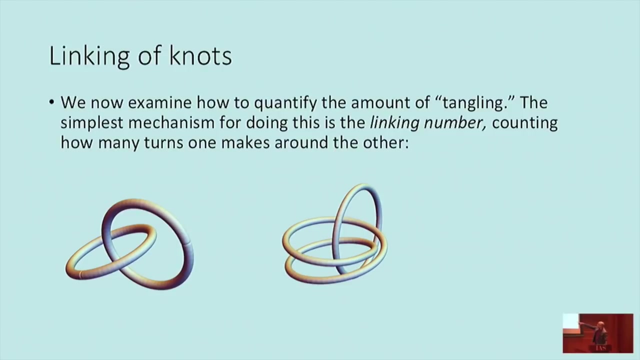 and I want to know how tangled are they? There's one very simple measure of it, which is called the linking number. okay, And I will just explain this by picture. So in this picture on the left, the horizontal knot winds once around the vertical one. 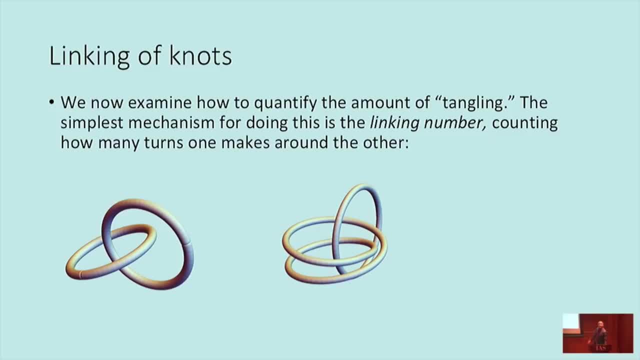 The picture on the right, it goes twice around. okay, And so we say the linking number in the first case is one and the linking number in the second case is two. So it's a bit tricky to define this mathematically. 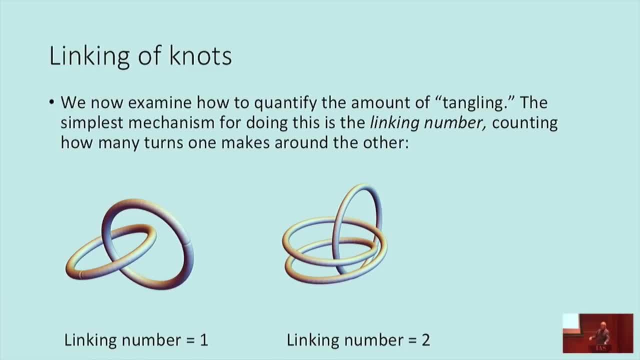 but you know, if you make this physically, you know with something like these glow sticks, you'll immediately see there's a huge difference between the two. There's much more tension in the second case than the first case, So they're very, very different. 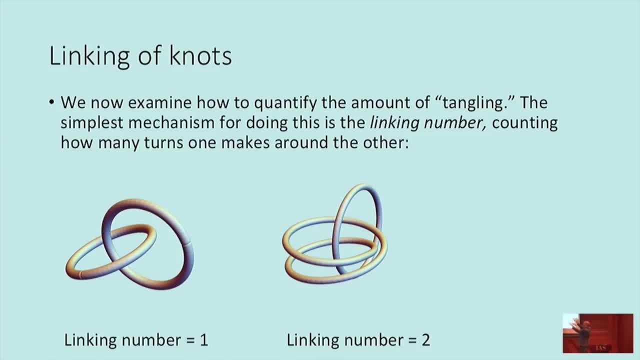 So this is very So. without giving you the mathematical definition, it just You count how many times one goes around the other. Now I want to describe what the analog is at theconcerning factorization, And this requires me to set up a little. 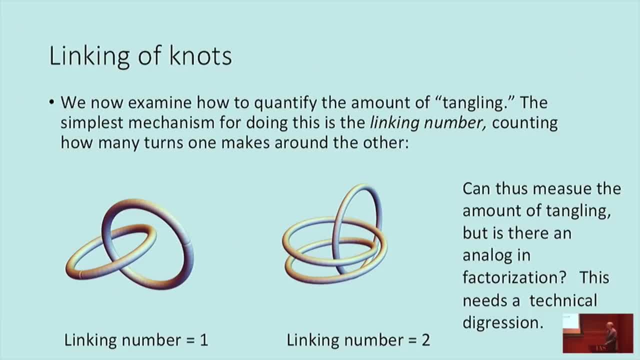 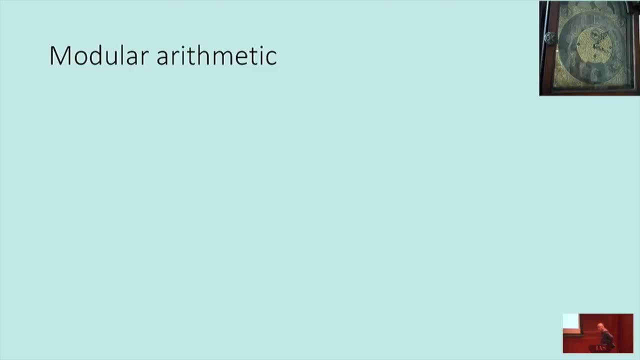 to be a little bit technical for the next couple of slides, But if you get lost it will, Don't worry, it will, It will end, Okay. so I'm going to tell you about a little bit about modular arithmetic. 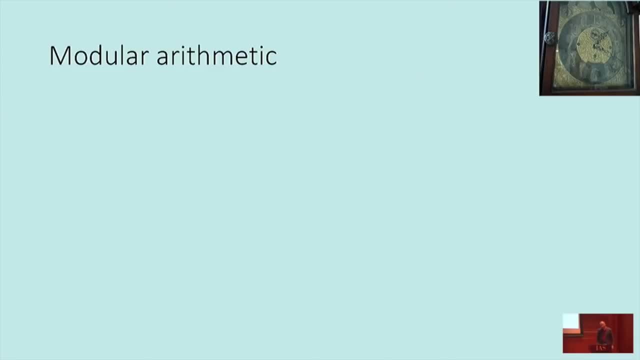 All this is for the purpose of describing, in the end, what the analog of I mean. does it make sense to say that two prime numbers are linked? So modular arithmetic. it's a kind of a toy version of arithmetic And it works like 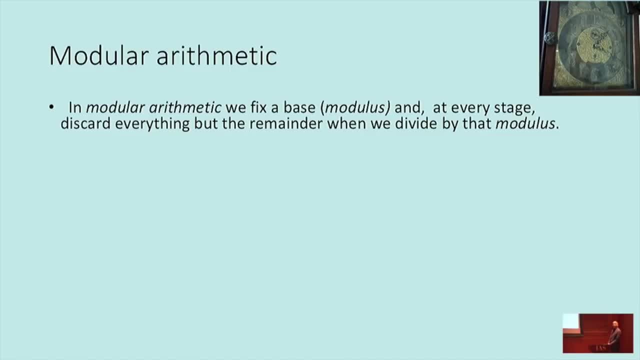 I'll tell you the rules of the game. You fix a base which is called a modulus. Okay, so just Let's say that modulus was 10. And the rules of modular arithmetic are: There are whole numbers involved. You do arithmetic, as usual, with those numbers. 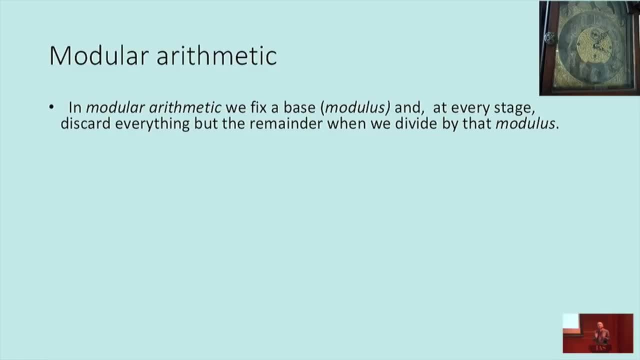 But at the end of every operation you discard everything except the remainder when you divide by the modulus. Okay, so I'm going to give you several examples to talk through that. So let's start with modulus 10.. So in modular arithmetic, with modulus 10,, 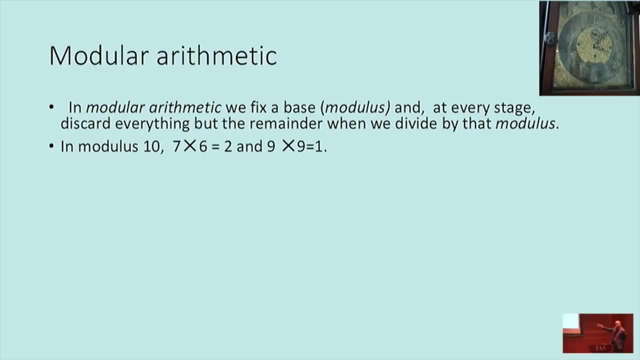 if you want to work out 7 times 6, you work it out as usual: It's 42.. But then you divide it by 10. And you see the remainder is 2. And so you just forget the rest. 7 times 6 is equal to 2 in the system of arithmetic. 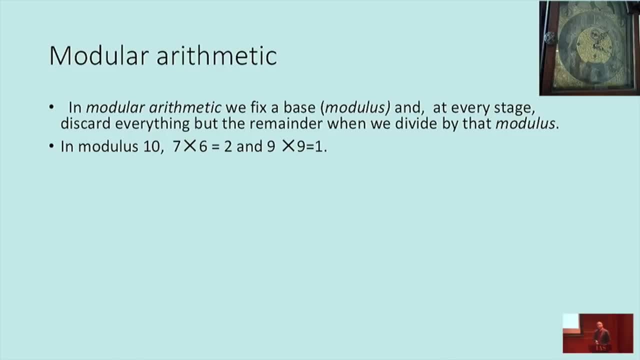 9 times 9 would normally be 81. When you divide by 10, the remainder is 1.. So you say 9 times 9 is equal to 1.. So, as you can see, this is in general simpler than ordinary arithmetic. 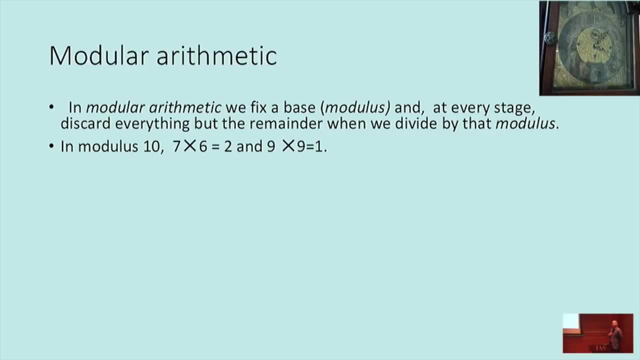 because this process makes the numbers much smaller. Okay, after you take the remainder, it cuts the large number down. I'll give you a couple more examples. So in modulus 7, 3 times 3 is equal to 2.. And the reason is it would ordinarily be equal to 9.. 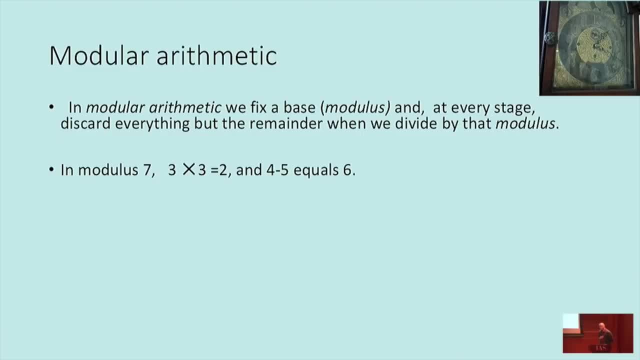 But when you divide it by 7, it leaves a remainder of 2.. And 4 minus 5 is equal to 6, which I'll leave you to think about. So this- although I've sort of said this in a way that makes it look exotic- 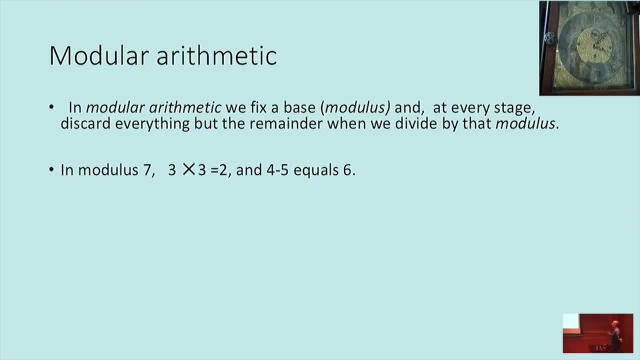 but this is actually something that we do very naturally when we think about cyclical things like time. Okay, so if I say to you that something happens 17 hours after midnight, you would translate it in your mind to 5 o'clock, And all you're doing is you're subtracting. 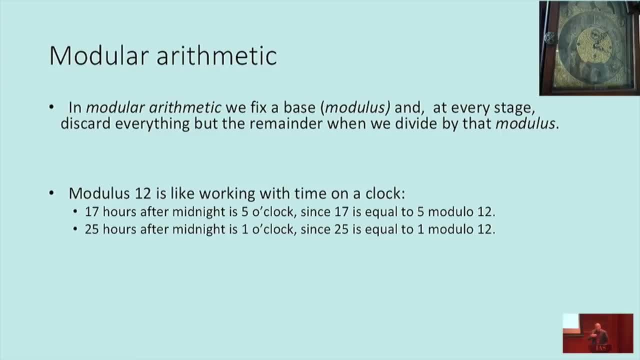 you're dividing by 12 and just keeping track of the remainder, which is 5.. Okay, So when you do modular, a lot of things you do just when you work with time, are, in mathematical terms, working modulus in modulus 12.. 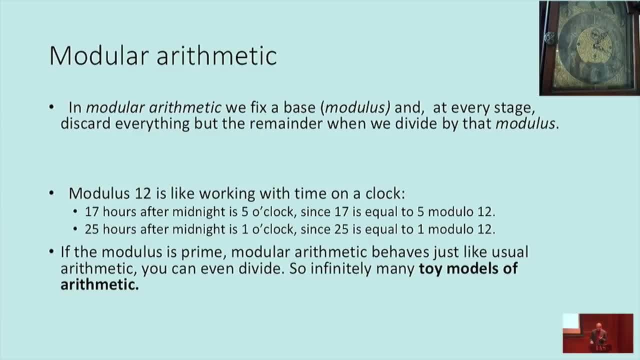 So the way to think of this is: for each modulus you have this little toy model of arithmetic. Okay, if that modulus happens to be prime. so if you do modular arithmetic, modulus 29,. it behaves in every way like ordinary arithmetic: You can add, subtract, 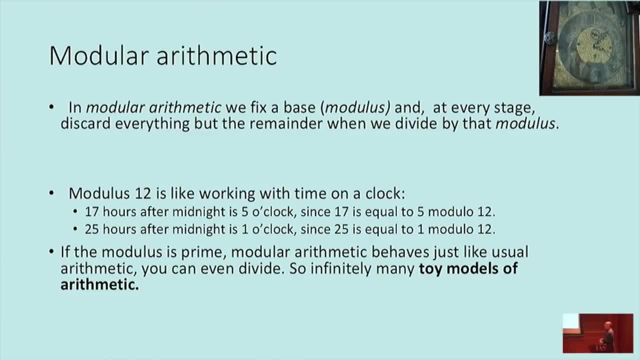 multiply and you can even divide And it satisfies all the rules that you know from ordinary arithmetic. So it's like a little toy model of arithmetic And you have one for each modulus. Okay, so you have these infinitely many little models of arithmetic. 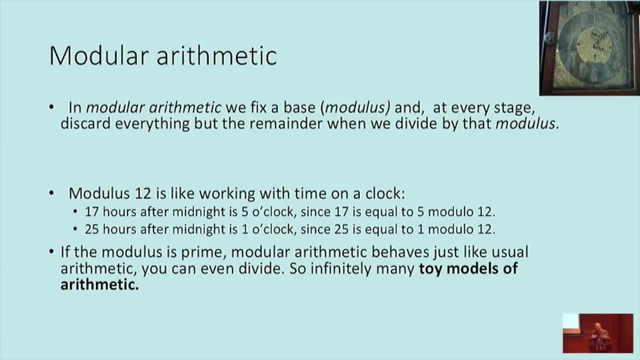 They're extremely useful in number theory because, as I said, many problems become simpler. The one thing I maybe emphasize about them is that they are to a very, very good approximation. they behave completely as if they're completely independent. Okay, so if you do, on the one hand, 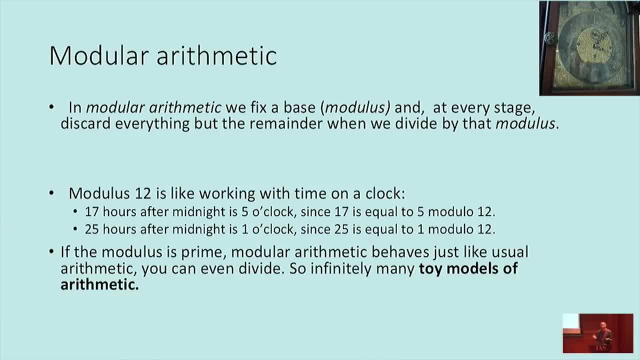 modular arithmetic to the modulus 29 and modular arithmetic to the modulus 31,. they really don't know anything about each other. Okay, they're completely different things, Okay. so I said most problems are easier in modular arithmetic, Not all, And I'll give you the simplest example of one. 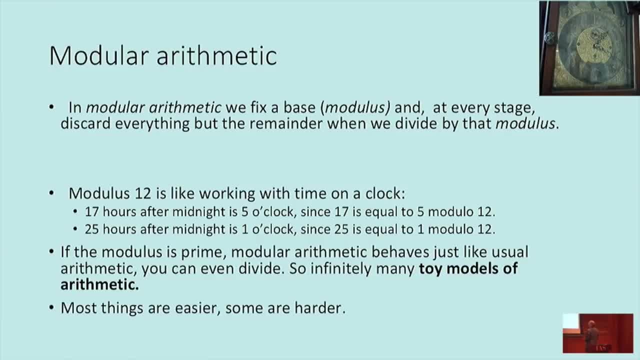 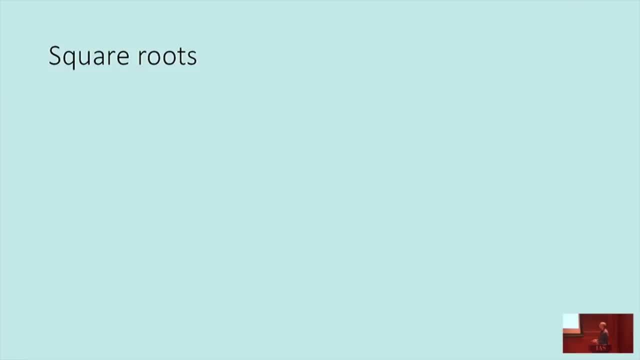 that is not okay. So this is the problem of taking square roots. So in ordinary arithmetic, in fact, I'm not even going to talk about taking square roots, but just which numbers have and don't have square roots. So if you deal with ordinary arithmetic, 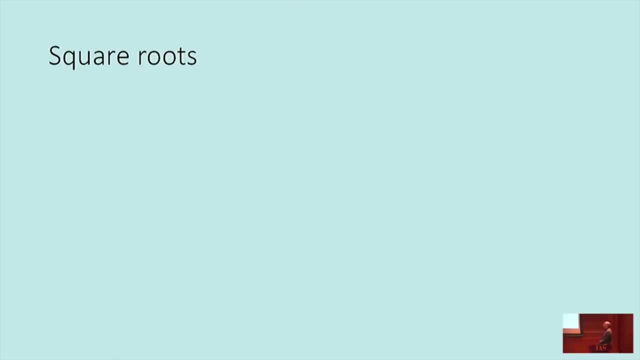 and not just whole numbers, but you allow decimals. it is very easy to know which numbers have square roots and which don't. The ones which have square roots are positive and the ones which don't are negative. Okay, so roughly speaking, 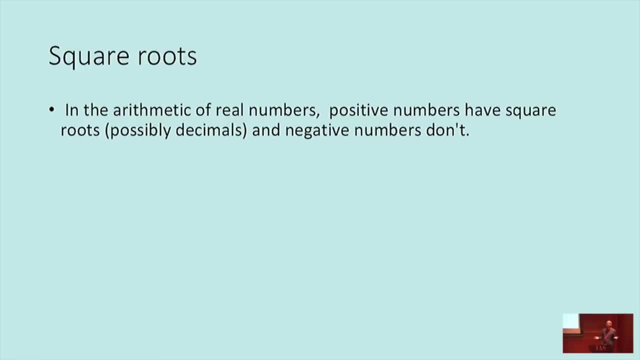 half the numbers have square roots and half don't, and it's easy to tell which has a square root if it doesn't have a minus in front of it. If you work, say, in modular arithmetic to the modulus 29,, it's again true that half the numbers 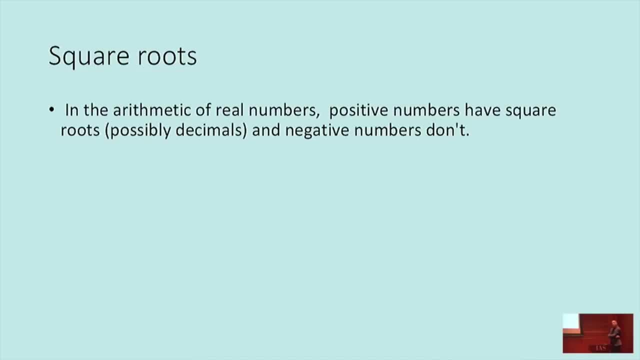 have square roots and half don't, but it's no longer apparent which is which Okay. So just to give you an example to Modula 7, in Modula 7, 3 times 3 is equal to 2.. 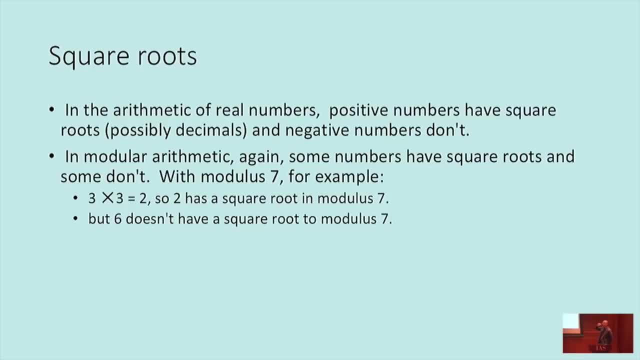 I said that on the last slide It would be 9,, but the remainder is 2.. So in other words, in Modula 7, 3 squared is equal to 2.. So 2 has a square root. On the other hand, 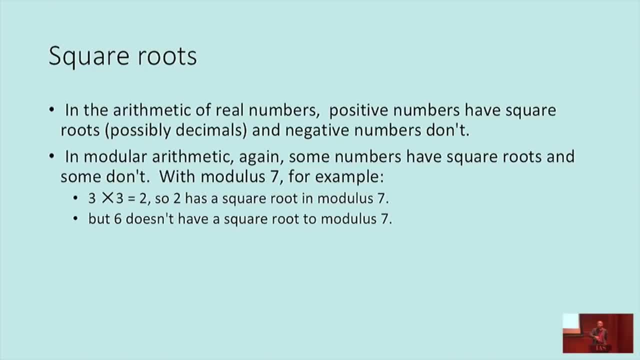 6 doesn't have a square root in Modula 7.. So you can go and take a look at this. So you can go and take 1 times 1,, 2 times 2,, 3 times 3.. You will never hit 6.. 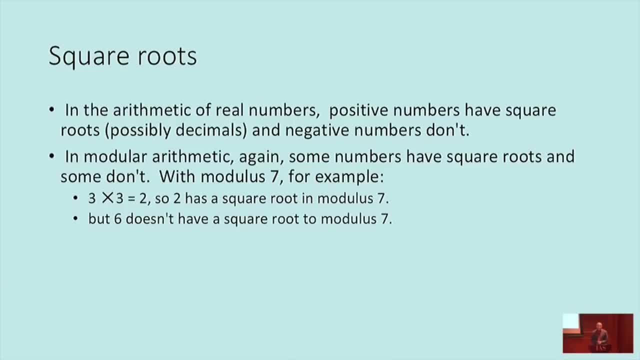 So some numbers have square roots, some don't, but the difference is that it's sort of hard. 2 is in this system of arithmetic like a positive number. 6 is like a negative number. But it's not so easy by looking at them. 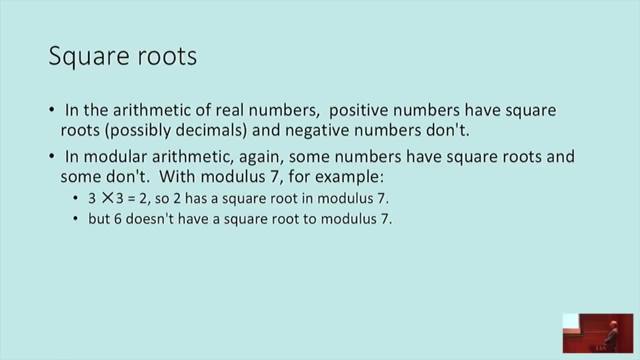 to tell which was which Okay. so, for example, if I ask you a question like does 5 have a square root in Modulus 3001?, You know you would have to start multiplying and it's not so easy to tell. 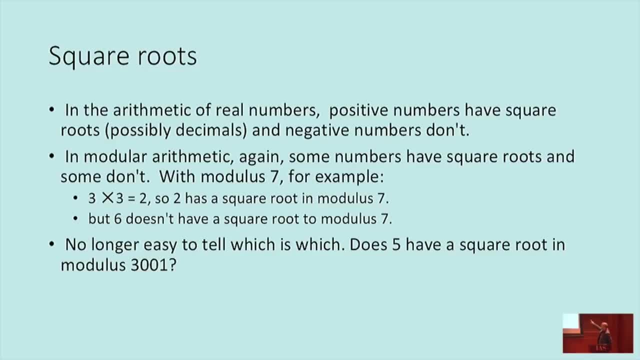 Okay, so I'm not going to come back to this, but I will say if you pay attention to the next few slides, I will say enough to solve this problem. So if you enjoy such things, you can come back to it and see if you can figure it out after two slides. 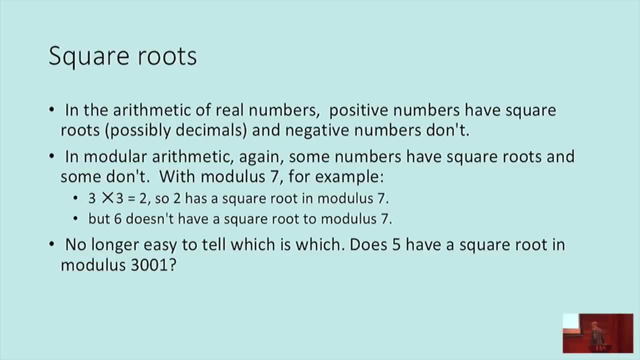 Okay, so all this, as I said, so square roots in Modula are things that in regular arithmetic- unlike regular arithmetic- are not. it's not even simple to understand which numbers are, so to speak, positive or negative, And I talked about this. 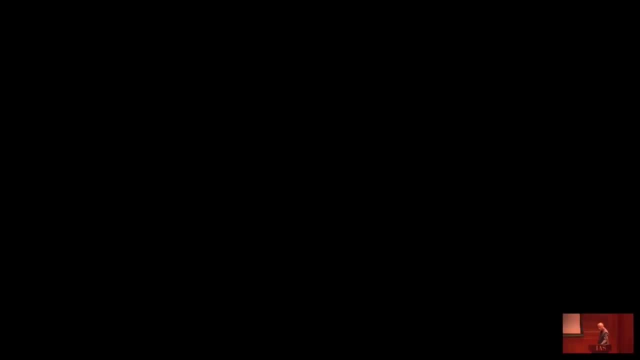 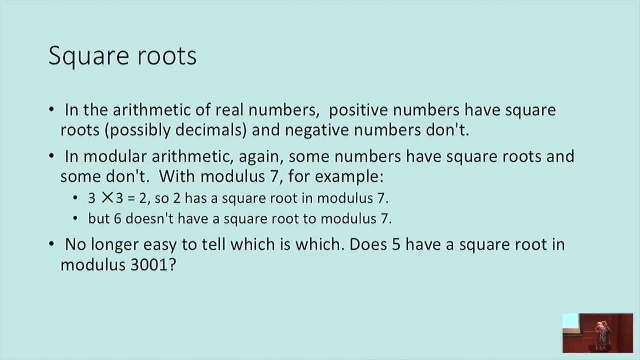 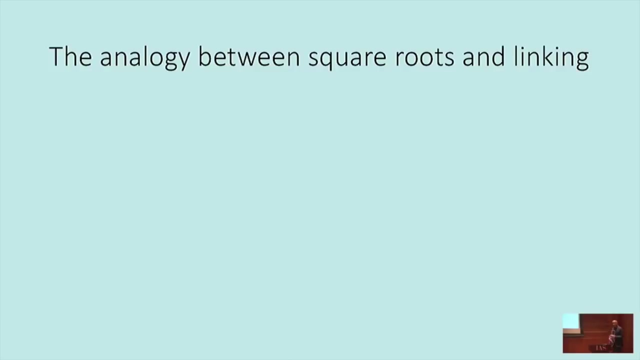 because I was trying to describe what the oops. no, that wasn't good. Okay, there we go. I was trying to describe what the analog of linking was for the linking between two knots in number theory. Okay, so let me describe. 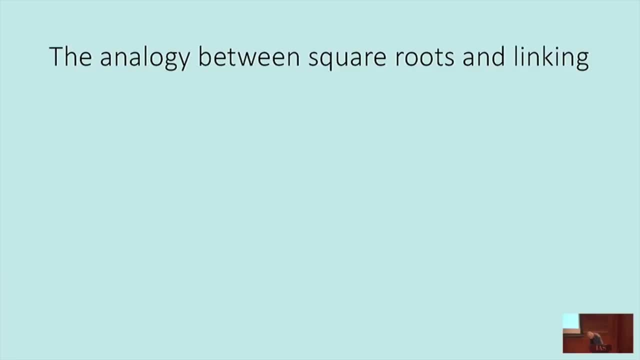 I will describe for you the analogy, And so this I'm going to, okay, I'm going to try to tell you something in number theory that is analogous to linking. Now, it's not, it's not a perfect analogy, in that it's not. 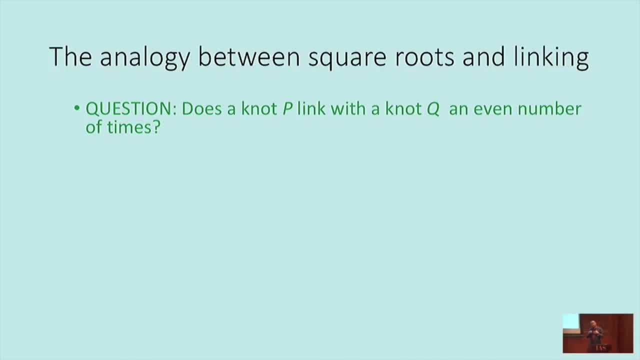 there's no analog available for exactly what is the linking number of two knots, But I'm going to. if I ask it, does one knot link two knots With another an even or odd number of times? Okay, that is. I forget whether it links. 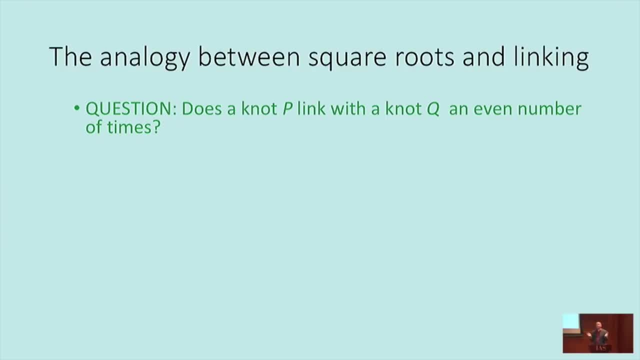 that linking number is. it winds around the other seven times or eight times, I just remember. is it odd? or even We understand a very good analog of that question for primes. Okay, and this is it's. there is a. 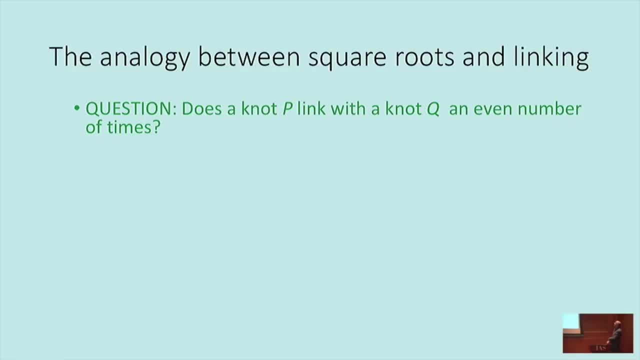 this does come from somewhere, but it's not easy for me to motivate, so I just ask that you take it on on faith for the moment. We'll see what it implies. This question: does a knot, does one knot, link with each other, even or oddly? 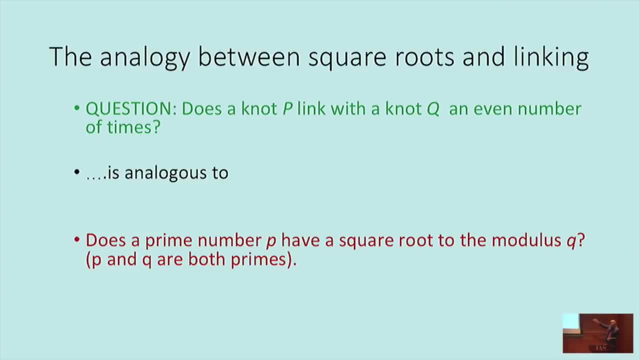 It's analogous to: does one prime number have a square root to the modulus of another prime number? So, for example, if the primes were 29 and 17,, I would be asking: does 29 have a square root in modulus 17?? 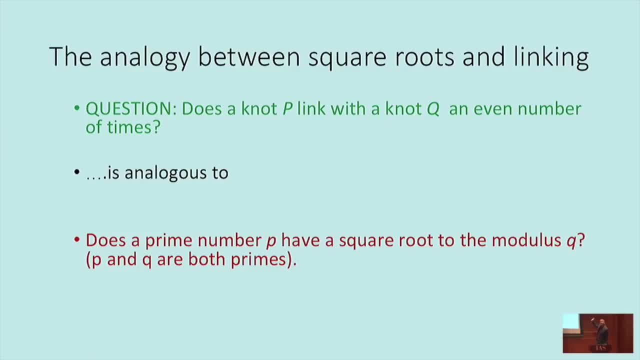 This is a yes- no question. Okay, the answer to the bottom is either yes or no. Yes is meant to be, yes is meant to be the analog of even and no is meant to be the analog of odd. So let's accept that for a moment. 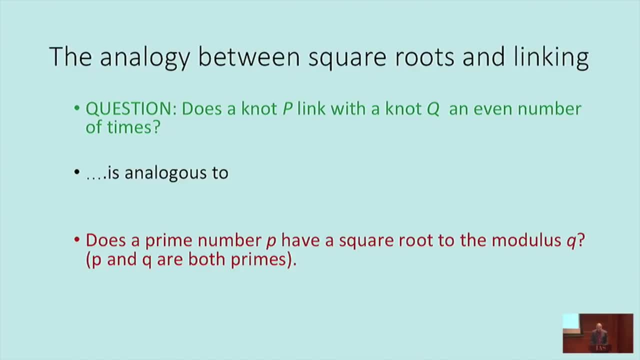 In fact, you just have to accept it. I'm not going to explain it, But I want to tell you, then, something very remarkable that it implies: Okay, so if you believe that these things are analogous, it tells you something which is very surprising. 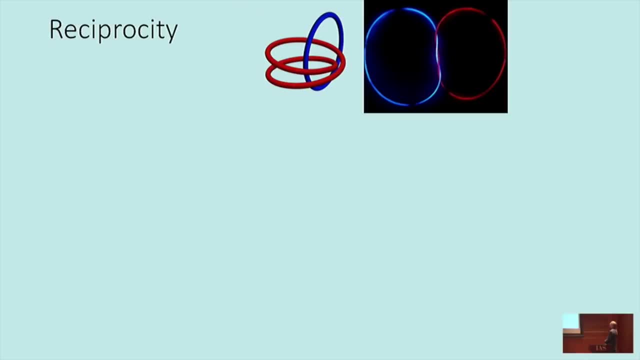 So I didn't really make a big deal of this. This is the diagram I showed you when I talked about linking number on the left, But this notion of linking number is completely symmetrical. Okay, that is, if you make this, you know if you make. 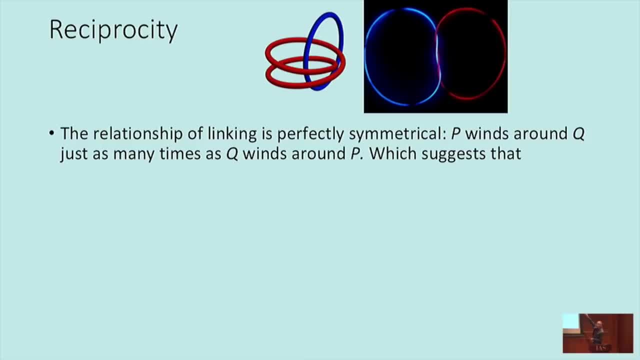 I made this thing with my glow sticks and it snaps into this configuration on the right. Okay, and it's very clear that the red one winds around the blue one exactly as many times the blue one winds around the red one. Okay, so either way, 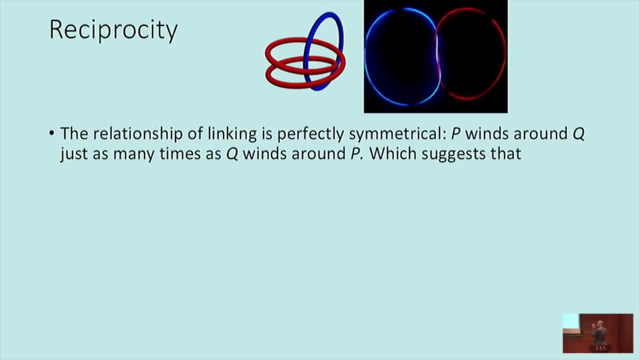 you can think of it from the point of view of red going around blue or blue going around red. They're exactly the same Either way, the linking number is two. Now, if you believe my analogy, it then says that the same should be true. 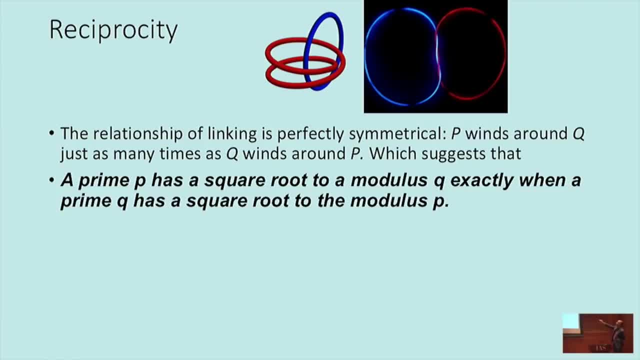 for prime numbers. That is a prime number, so let me just say it with 17 and 29.. So 17 will have a square root to modulus 29,, exactly when the other way is true, 29 has a square root to modulus 17.. 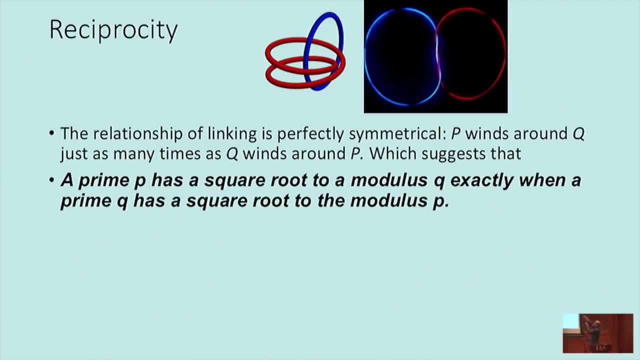 Now, you know, since you've just seen this concept, I think it's hard to sort of appreciate what a strange type of assertion this is. And the reason is that, as I said, with 17 and 29, arithmetic modulus 17. 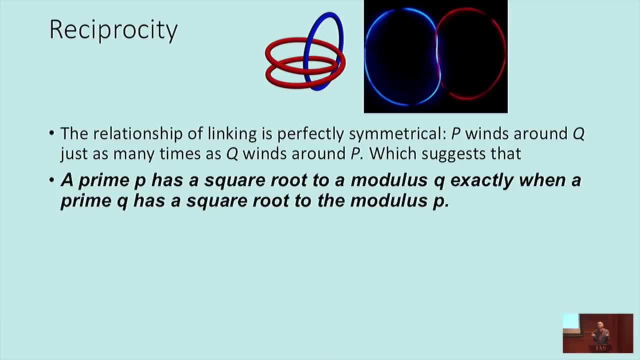 and arithmetic to the modulus 29 are completely different. They're completely different worlds. Okay, so whatever the nature of this statement, it is some link between these toy models of arithmetic, and this is a very surprising thing. Okay, it's true. 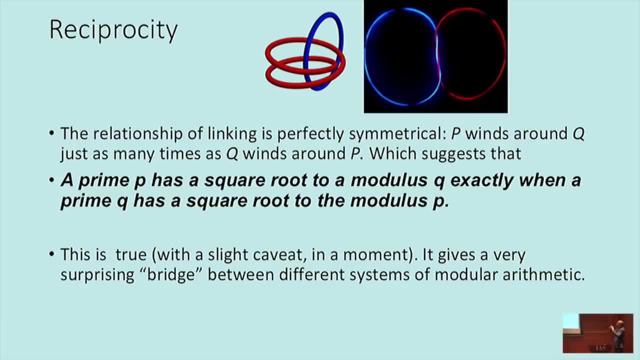 and I'll tell you exactly what's true in just one moment. but, as I said, what's surprising it's a bridge between these two different systems of arithmetic which in most ways, as I said before, are completely unrelated. Okay, so this statement, 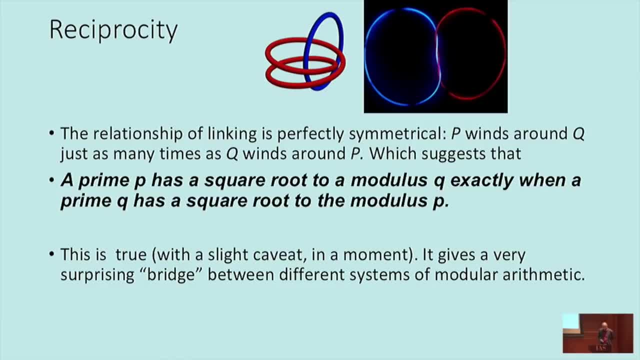 I said at the start of the talk, I would tell you the two things you would encounter in an undergraduate course on number theory. This is the second one and it's really in some ways, the sort of start of modern number theory. 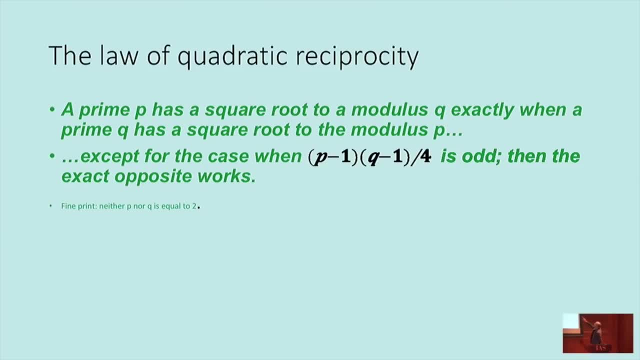 Okay, it's called quadratic reciprocity. I'm sorry about the font here, So what it says is exactly what I said on the last slide. if you have two primes, one has a square root to the other modulus, when this is a square root in this modulus. 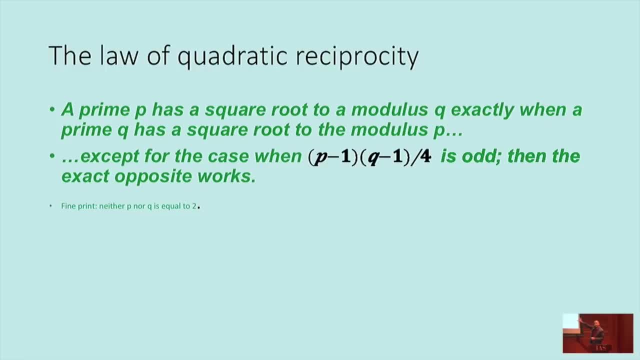 except there is an exceptional case which behaves in exactly the opposite way, That is to say, if p has a square root to modulus q, then q doesn't have a square root to modulus p, and vice versa, So they're still perfectly correlated. 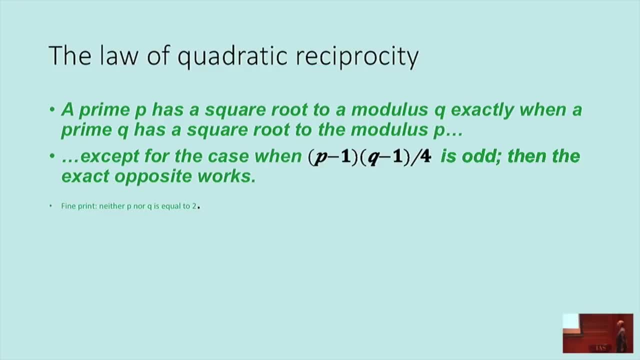 but it's just the exact opposite. Okay, and there's some fine print about this, which, fortunately, you can't read, so it's fine. Okay, this is called the law of quadratic reciprocity. It was proven by Gauss when he was 21.. 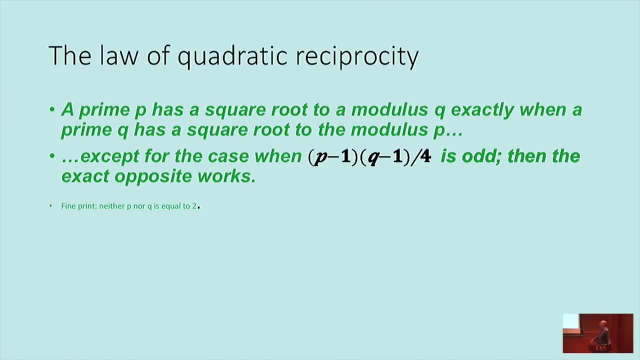 He was very proud of it, I think, exactly because it's extremely surprising. It connects two things that have no right to be connected And, again, the The fact that it's not Notice. this analogy did not work perfectly. Okay, there was this case. 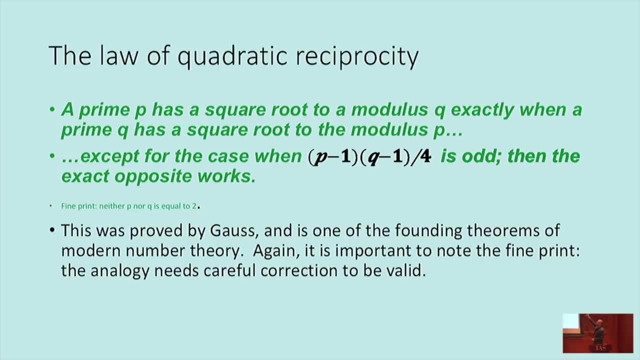 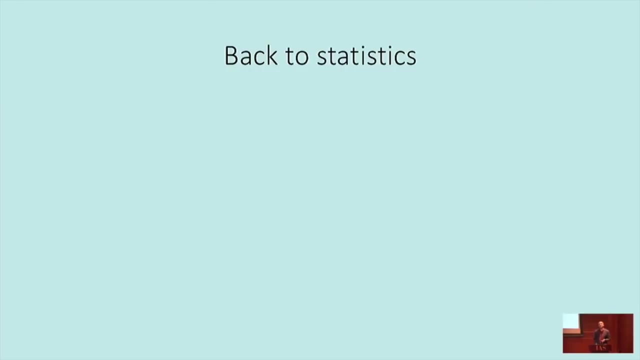 which worked in exactly the opposite way. So the statement is very similar to the fact that the linking of two knots is symmetrical, but you have to know exactly how to correct it, And that's again important. Okay, So now let's go back briefly to statistics. 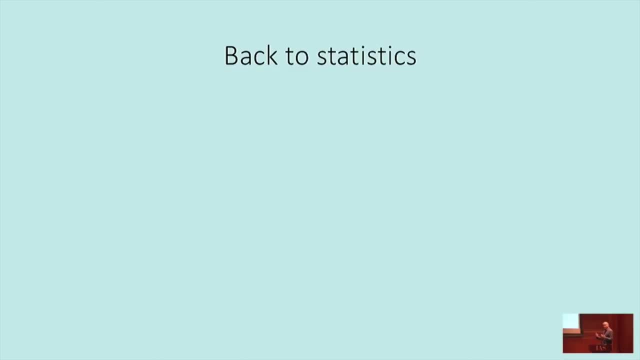 So the reason I was talking about this to start with was that initially, I took a number. On the one hand, I took a number and factored it. On the other hand, I made this tangle and I said that the factorization is analogous. 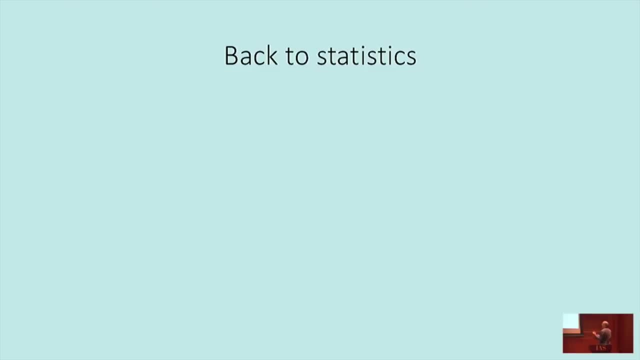 to this tangling. Now I have sort of a way that I can measure the On one side. I can measure the linking between different pieces in my tangle On, That's on the side of the, On knots, On the side of numbers. 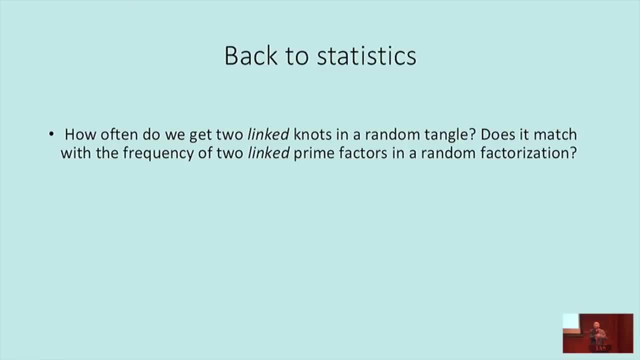 I can If I have two prime numbers. I have this Now. I have this notion of whether they're linked or not by measuring whether one has a square root in the other modulus. Okay, And now you? So you can start to think about statistics of that. 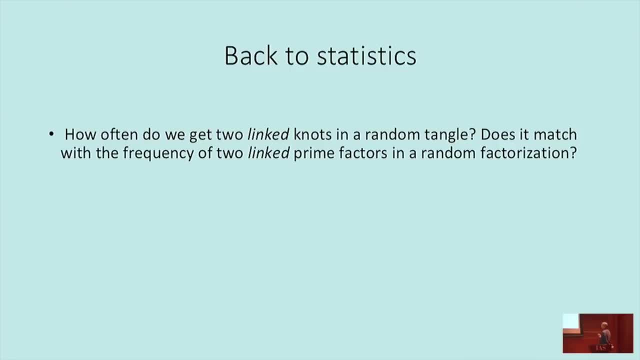 and ask whether they're the same, And So this question is. It's actually. This type of question is a topic of active study, and it's subsumed in a sort of more precise question. So there are. So mathematicians keep track of objects. 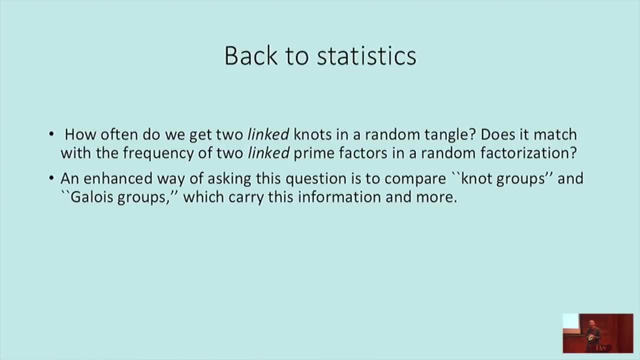 that carry more information than just these linking numbers. So if I have one of my tangles, I can look at something called its knot group or its link group, which keeps track of all the linking numbers, but it also keeps track of more information. 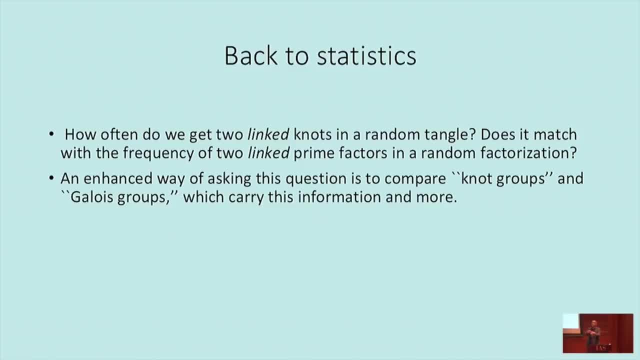 For example it keeps track of There are ways in which three knots can be linked without any two of them being individually linked, and so on. So that type of information is carried in this thing called the knot group On the number theory side. 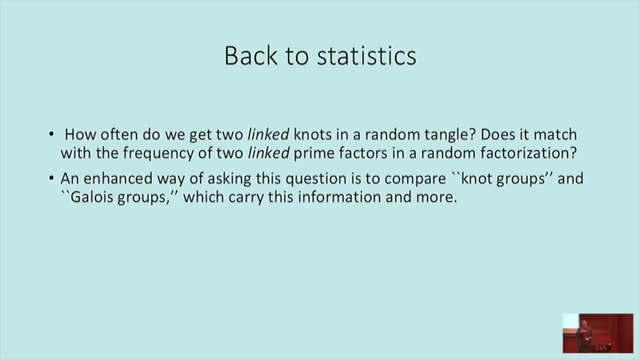 there's an analogue of that which is called the Galois group, or the unramified Galois group, which keeps track of the information of whether all these prime factors are linked. Okay, And in the last 20 years or so, there's emerged a field of number theory. 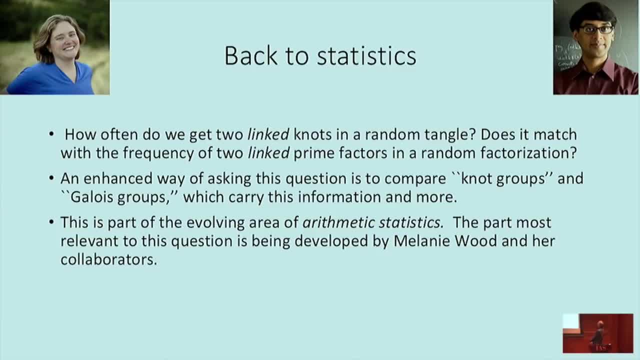 which was essentially, I would say, founded by Manjul Bhargava in his thesis called arithmetic statistics, which, a very kind of exciting part of this field, studies exactly this question. okay, Are the behavior of these knot groups and Galois groups the same? 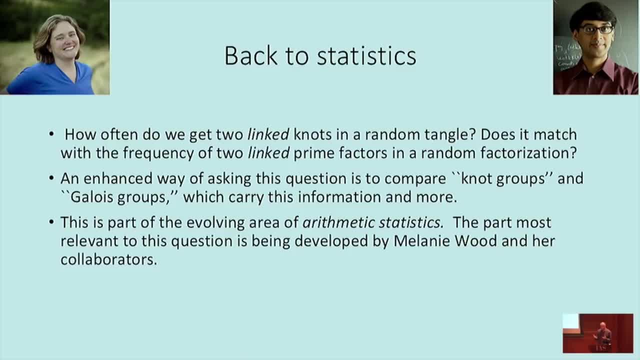 Which you can think of as an enhancement of the statistical questions I was asking before, but now keeping track of this tangling information. Okay, And so the part which is most relevant to that is being studied by Melanie Wood, whose picture on the left. 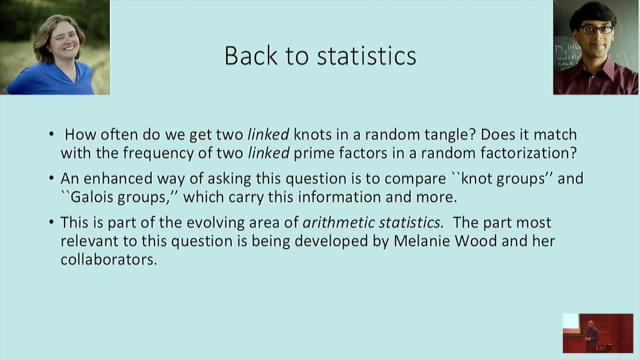 So I want to say a bit about this, because so arithmetic statistics is the part of number theory which studies statistics. you do something like factorize, you do it many times and you see what happens. You study the statistics of what happens. 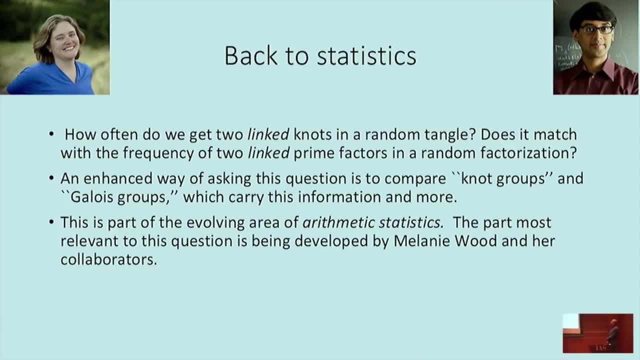 And this I think it's a very powerful way of looking at this. You see, this analogy between primes and knots is a little bit vague, or historically has been a little bit vague. That is, there are concepts on one side and concepts on the other side. 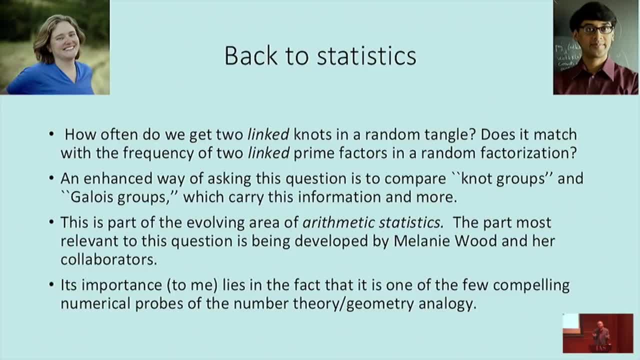 and they look like one another. But looking like that is a bit vague for a mathematician. It's very hard to build on statements until they have acquired a certain degree of precision. Now this idea of looking at statistics of both sides, 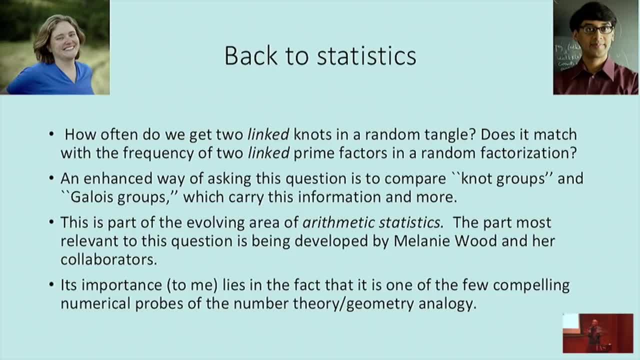 it really allows us to get to the point where we can make numerical measurements and we can demand they be equal. And I think in the process of that, we're seeing now that this analogy will become more precise because this, you know, taking statistics of both sides. 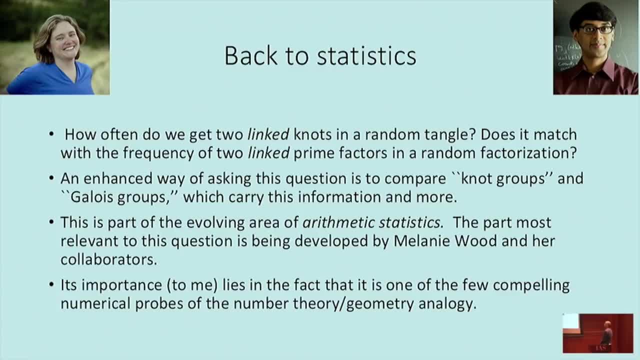 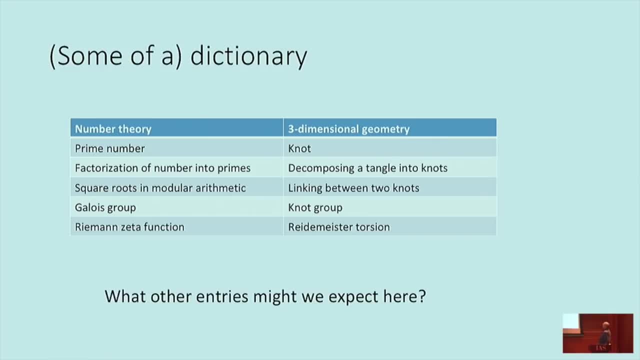 gives us really a way to test it in new and interesting ways. Okay, So here is. let me just recap what I've talked about on the side of, at least I've talked about, the first four entries in this table. primes and knots, factorization. 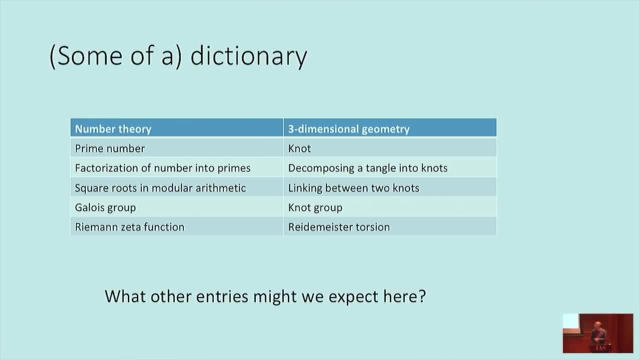 and decomposition of tangles, square roots and linking- and I mentioned Galois groups and knot groups. And I just want to finish with a little speculation about what we might hope for in the future of this table. Maybe before I say that I should say this is a pretty hard one, dictionary. 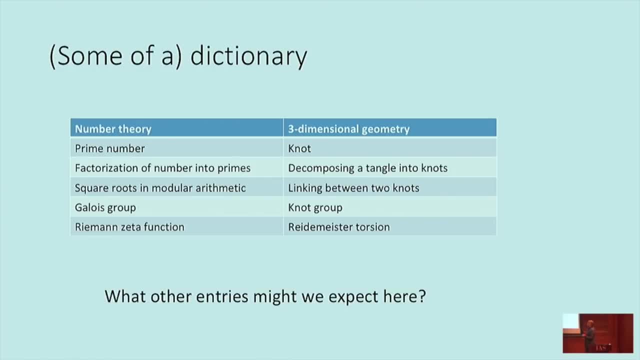 So it's the details. it's not so simple to take a concept on one side and, by pure thought, find what it is on the other. Okay, So it's the way, at least I see it. it's more that you have to already understand. 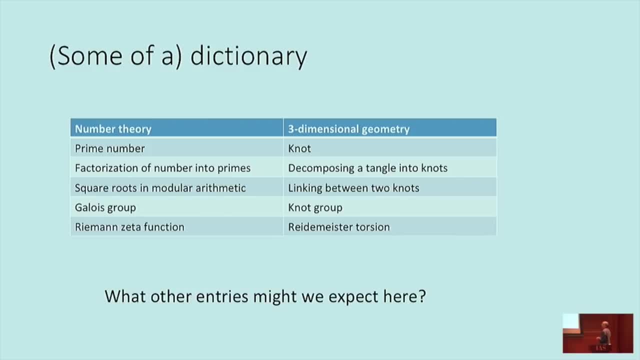 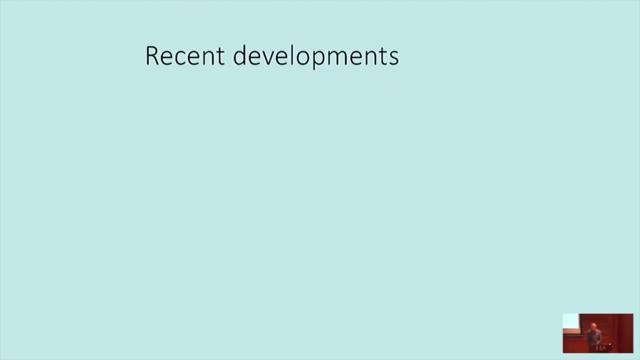 both things very well before you can see that they're analogous. So it's not this dictionary. it's maybe an art and not a science. But having said that, let me just say one more, one word about what we might hope for. 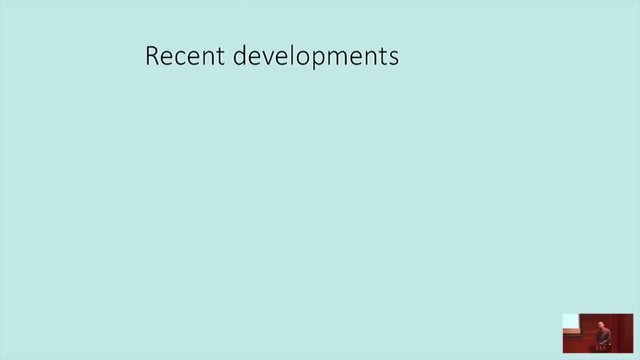 So everything I've talked about in knot theory on the side of knots is, you know more- a century old. It's been around for a long time linking numbers and all this. But knot theory was kind of from the mathematical point of view.